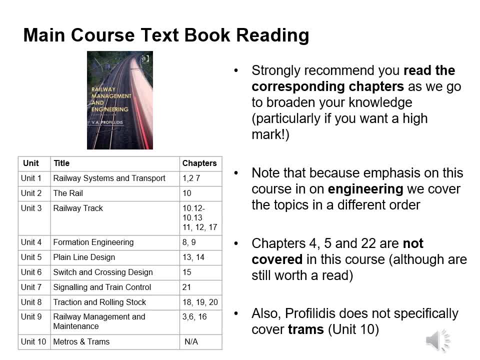 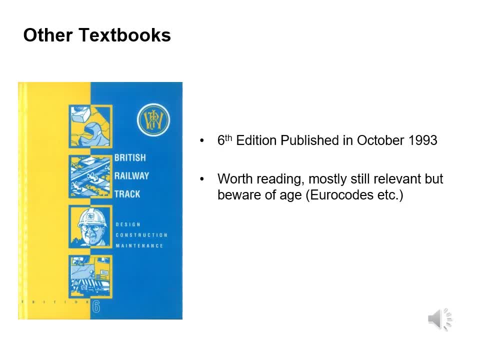 Also, the Profodilis does not specifically cover trams, unit 10.. I'm going to go through some of the other textbooks that I recommend, This one published by the PWI, British Railway Track Design Construction Maintenance. 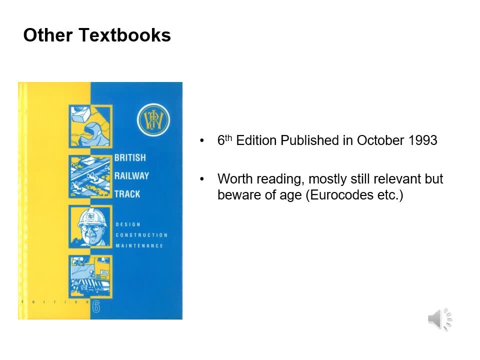 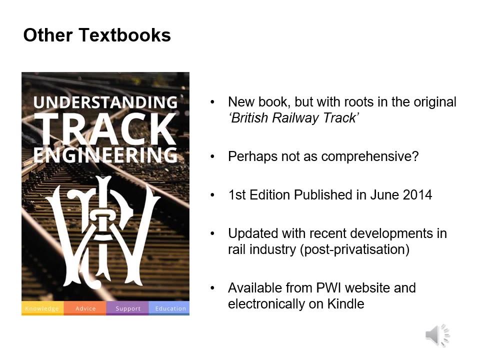 This is the sixth edition and it was published in October 1993.. It's well worth a read. Most of the content is still relevant, but be aware of the age, in particular reference to Eurocodes. This is the updated version of the PWI book. 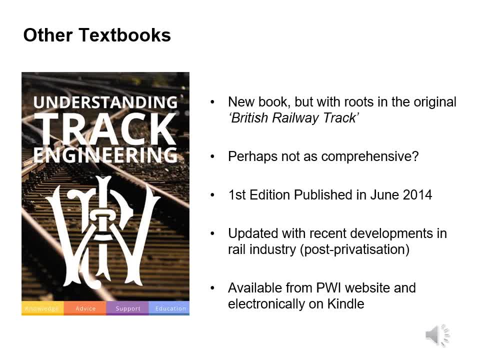 It has its roots in the original British Railway Track book, Perhaps not quite as comprehensive. I find the layout not as good And I find it somewhat lacking in technical content, So this first edition was published in June 2014.. It's updated with recent developments in the rail industry post privatisation. 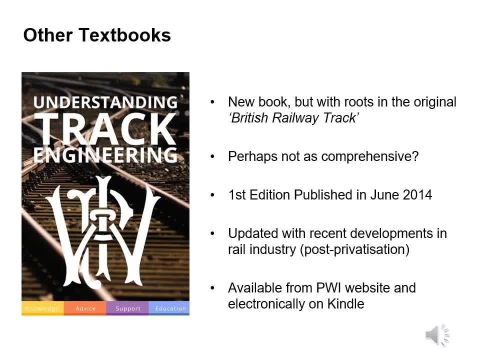 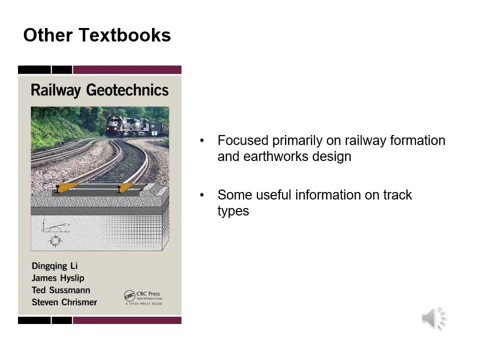 It's available from the PWI website and electronically on Kindle. So, as it says on the cover, Railway Geotechnics primarily focuses on railway formation and earthworks design. Some useful information on track types. If you're going to specialise in geotechnical engineering associated with the rail sector, then this is a highly recommended text. 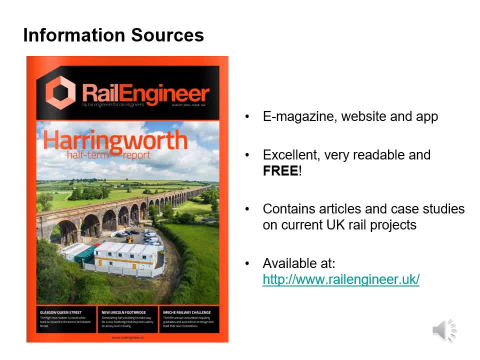 So Rail Engineer is probably the equivalent of New Civil Engineer for the railway sector. It's an e-magazine, website and app. It's an excellent publication, Very readable and it's completely free. It contains articles and case studies on all current UK rail projects. 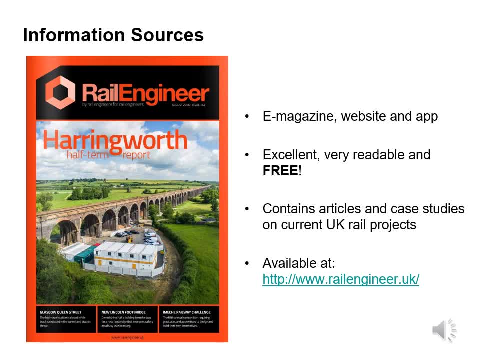 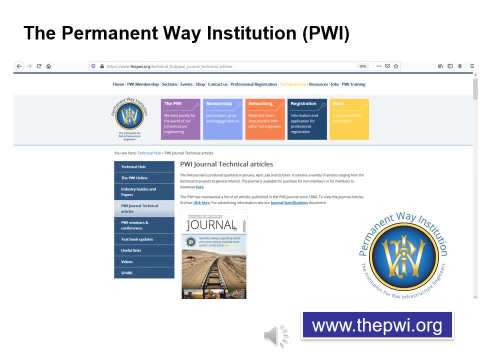 It's available at wwwrailengineeruk. Highly recommended. So if you're serious about becoming a railway engineer, you need to join the Permanent Way Institution or the PWI. This is the institution for rail infrastructure engineers and it's equivalent of the Institution of Civil Engineers for the railway sector. 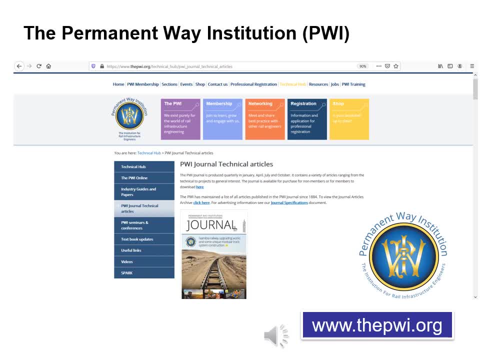 If you become a student member, which is free, you'll also get access to online version of the journal, the technical journal- that the PWI publish. This is a highly technical journal and has a wealth of technical information, Probably beyond the content of this course, but will prove to be quite inspirational and will help you on your way to becoming a professional railway engineer. 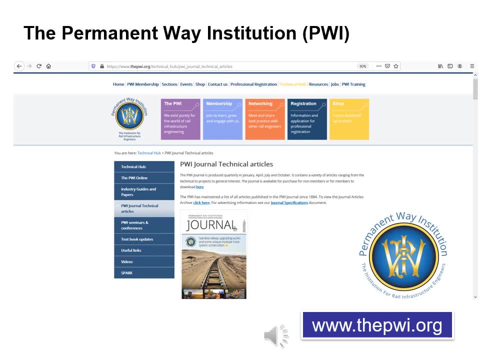 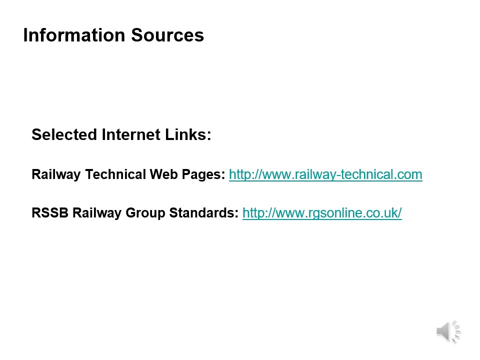 So get on the website, the pwiorg, and become a student member and get involved and go along to branch meetings. There's a wealth of information available on the internet, But these are two examples of internet sources that I recommend, The first being the railway technical web pages: railway-technicalcom. 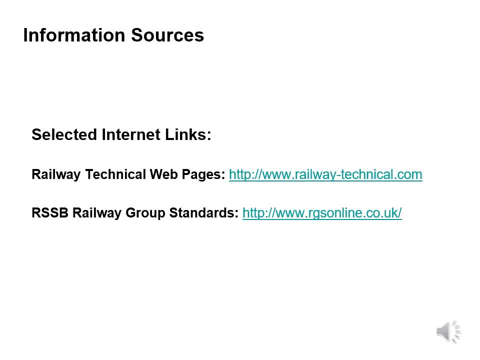 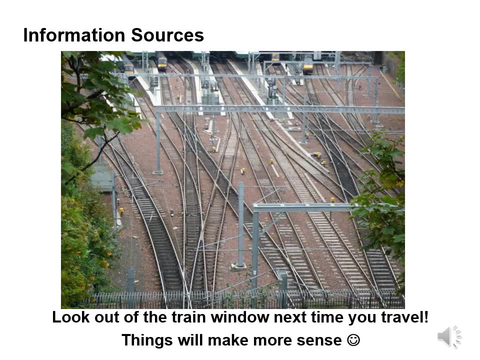 The second being the RSSB Railway Group Standards, which can be found at rgsonlinecouk. Next time you travel on the train, have a careful look out the window. A lot of what you'll hear about in this course will make much more sense if you observe it in real life. 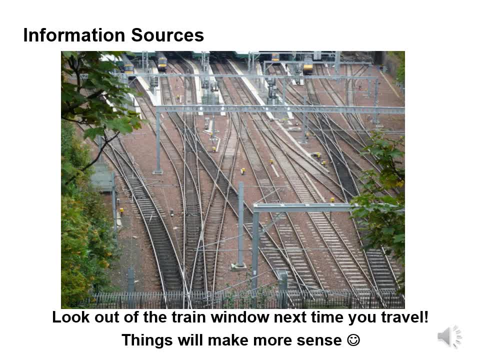 I'm going to present to you a range of videos which are going to show you some real infrastructure, which will help you understand the explanations I'm going to provide during the course. So when you get a chance, get out, get a ticket, get on the train. 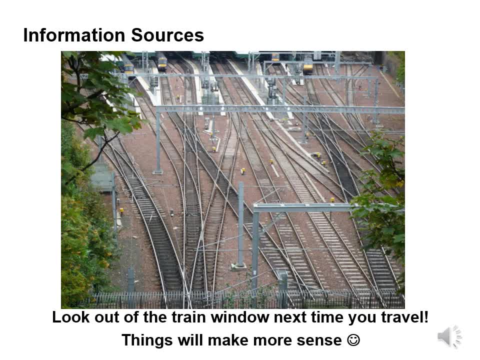 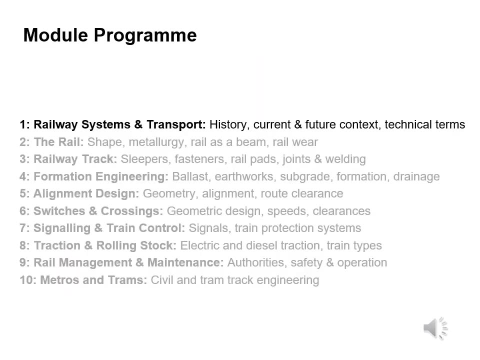 And, if you can, if you're in Edinburgh and you want a particularly special train journey, get a ticket to Inverkeithing and travel across the Forth Bridge. So Unit 1 of the module is going to look at railway systems and transport. 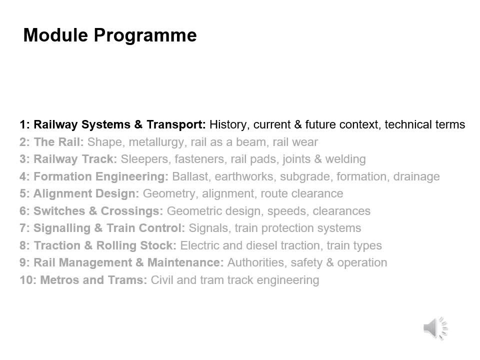 We're going to start off with a historical context. We're going to look at the current context in the UK and where we're going in the future, And I'm going to introduce some of the technical terms that you're going to use throughout the module. 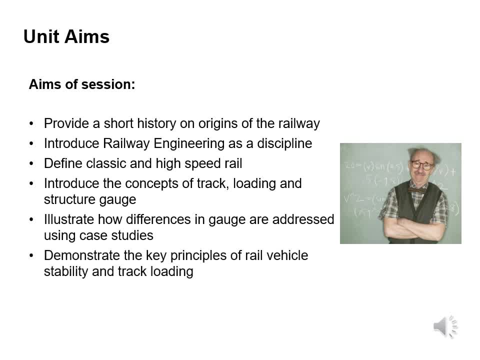 So in this unit, I'm going to provide a short history on the origins of the railway. I'm going to introduce railway engineering as a discipline. I'm going to define the difference between classic and high speed rail. I'm going to introduce the concepts of track loading and structure gauge. 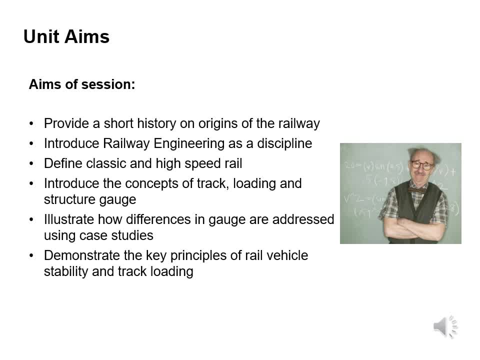 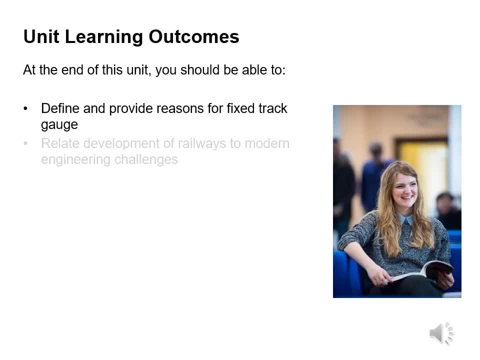 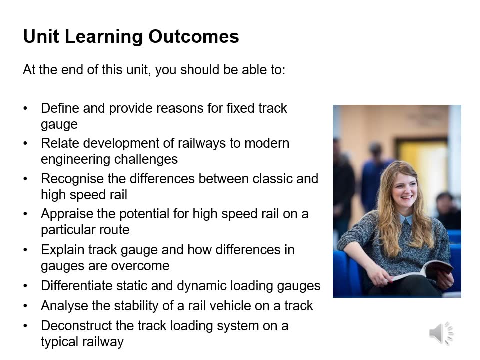 I'm going to illustrate how differences in gauge are addressed using case studies, And I'm going to demonstrate the key principles of rail vehicle stability and track loading. So at the end of this unit, you should be able to define and provide reasons for fixed track gauge. 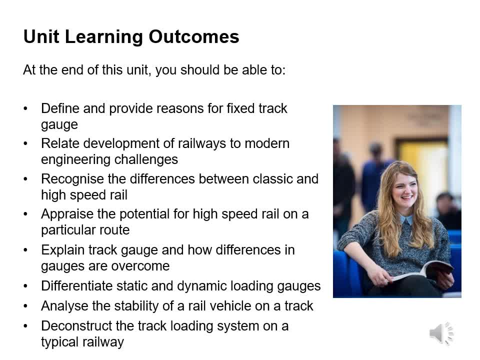 Relate development of railways to modern engineering challenges. Recognise the differences between classic and high speed rail. Appraise the potential for high speed rail on a particular route. Explain track gauge and how differences in gauges are overcome. Differentiate static and dynamic loading gauges. 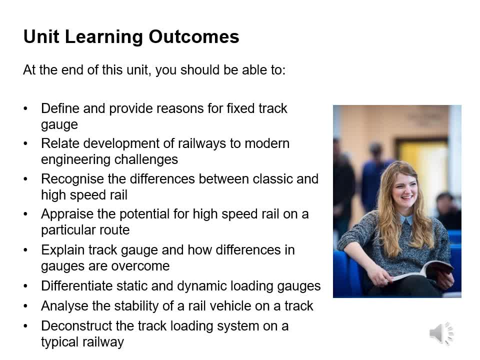 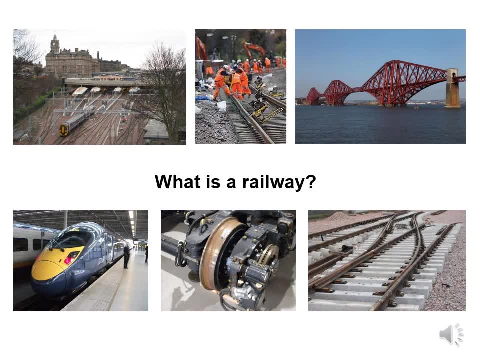 Analyse the stability of rail vehicle on a track And deconstruct the track loading system on a typical railway. So what is a railway? We're all familiar with trains and railways, But what is a railway? What is the definition of a railway? 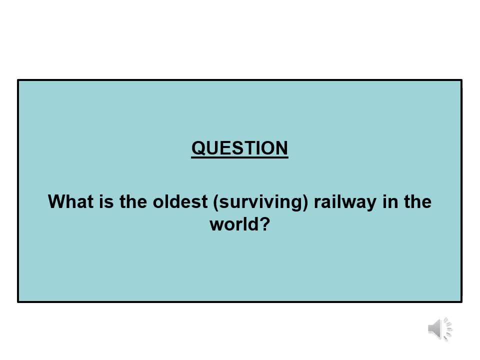 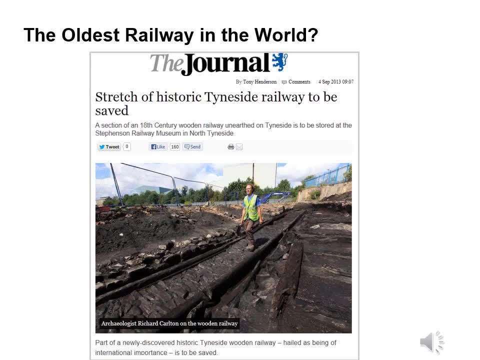 So my first question to you is: What is the oldest surviving railway in the world? In 2013,, archaeologists Alan Williams and Richard Carton discovered a wooden railway. This wagonway was constructed in the 1790s. They discovered a 25 metre long stretch of it. 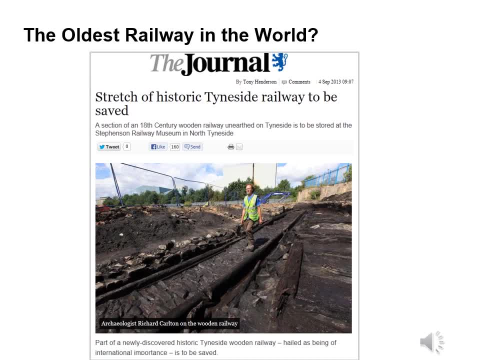 And it was at the site of the former Neptune shipyard in Walker, Newcastle. They discovered it as the site was being developed. The wooden track was used to carry coal from the collieries of Tyne for shipment. It is the earliest and the only surviving example of the standard gauge railway which spread across the world. 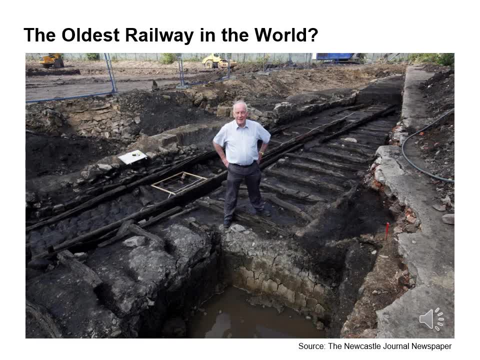 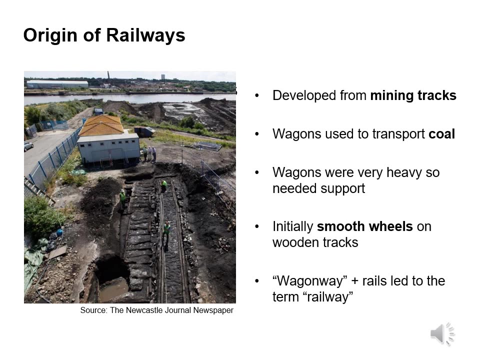 Here you can see a photograph of the railway Beautifully preserved in the ground. So the wagonway was developed from what was used in mining operations. The wagons were then used to transport the coal. The wagons were very heavy So they needed support. 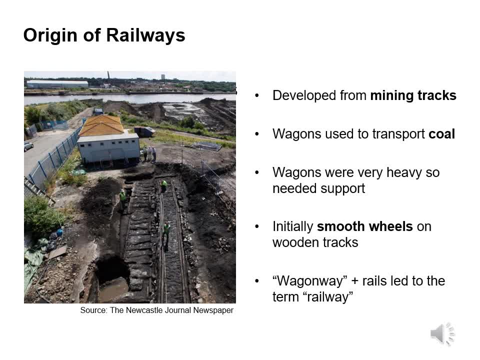 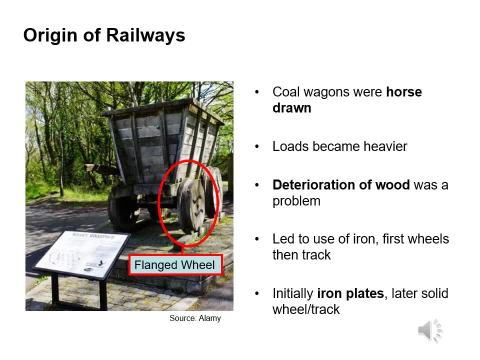 So initially smooth wheels and wooden tracks. So wagonway plus rails led to the term railway. So the early coal wagons were horse drawn and as the loads became heavier the deterioration of the wood became a problem And this led to the use of iron. 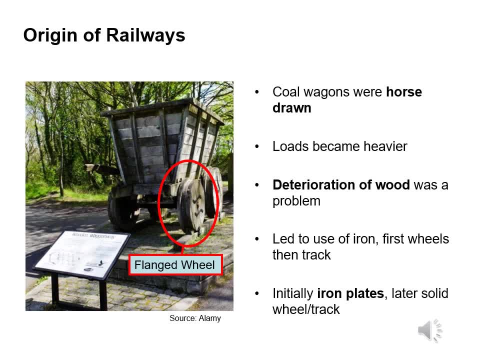 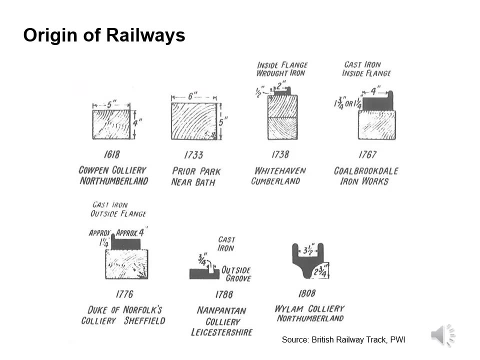 First the wheels and then the track. So initially they used iron plates and later solid wheels and track. And here you can see in this early wooden wagon That it actually has flanged wheels, Although they are still wooden. The introduction of steam engines for powering blast air to blast furnaces. 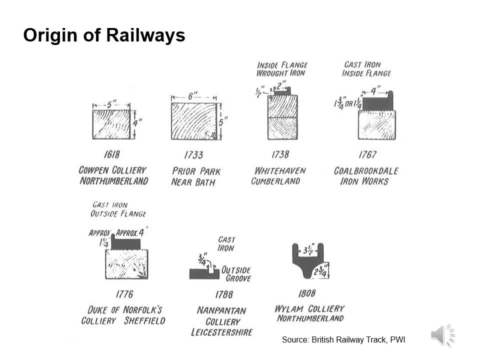 Led to a large increase in British iron production after the mid 1750s. In the late 1760s the Colebrookdale company began to fix plates of cast iron to the upper surface of wooden rails, Which increased their durability and load bearing ability. 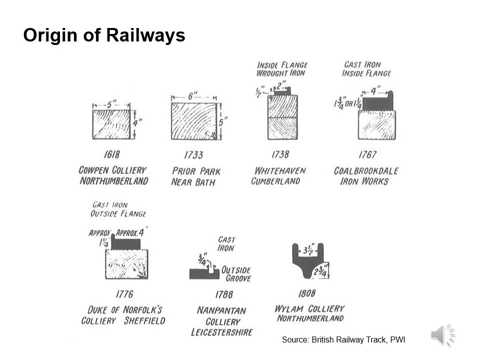 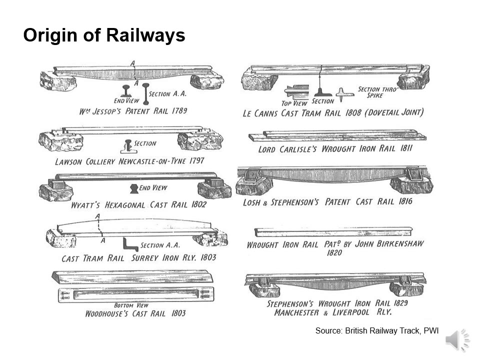 A system was introduced in which unflanged wheels Became iron L shaped metal plates. These became known as plateways. John Kerr, a Sheffield Colliery manager, invented the flanged rail in around 1787.. In 1789, William Jessop had introduced a form of all iron edge rail and flanged wheels. 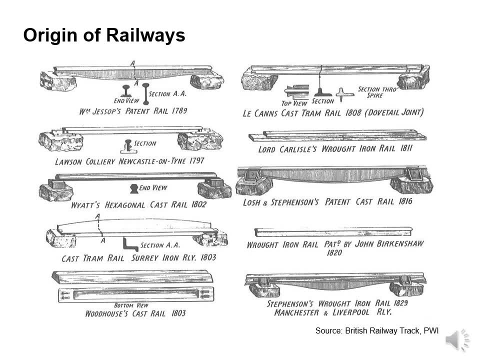 For an extension to the Charnwood Forest Canal at Nampanton, Loughborough, Leicestershire. In 1790 Jessop and his partner Outram began to build And began to manufacture edge rails. The first public edgeway was built by Lake Lough Railroad in 1796. 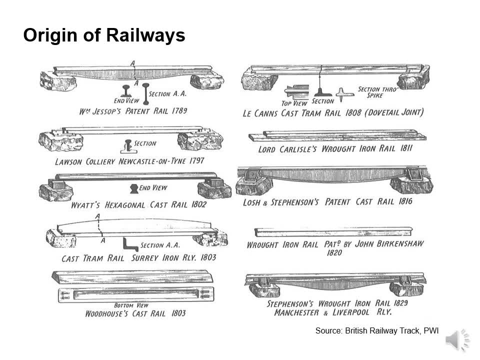 Although the primary purpose of this line was to carry coal, It also carried passengers. These two systems of constructing iron railways- The L plate rail and the smooth edge rail- Continued to exist side by side into the early 19th century. The flanged wheel and edge rail eventually proved its superiority and became the standard for railways. 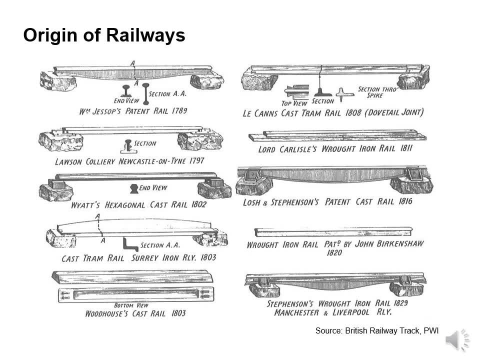 Cast iron was not a satisfactory material for rails Because it was brittle and broke under heavy loads. The wrought iron rail, invented by John Birkenshaw in 1820, solved these problems. Wrought iron, usually simply referred to as iron. 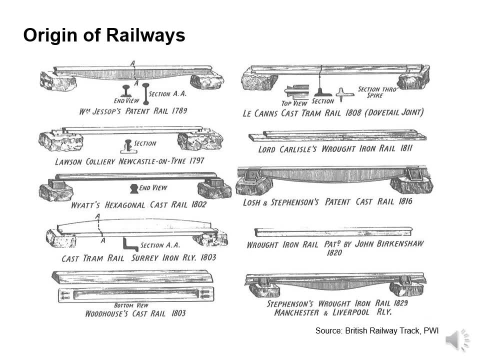 Was a ductile material that could undergo considerable deformation before breaking, Making it more suitable for iron rails. But wrought iron was expensive to produce Until Henry Cort patented the puddling process in 1784.. In 1783, Cort also patented the rolling process. 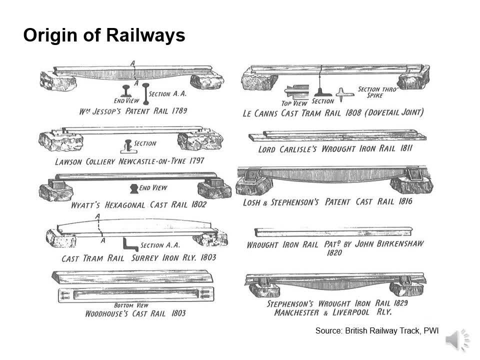 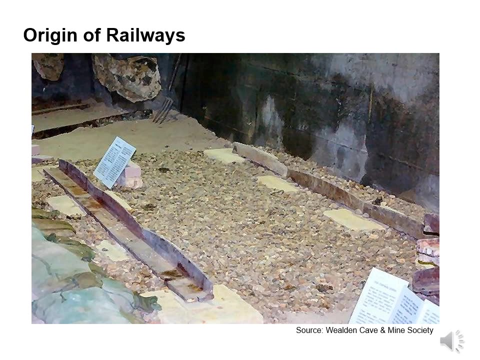 Which was 15 times faster at consolidating in shape in iron than hammering. These processes greatly lowered the cost of producing iron and iron rails. You can see from this image That the L shaped rails Are located on pads, But note that the rails are not constructed with sleepers connecting the rails together. 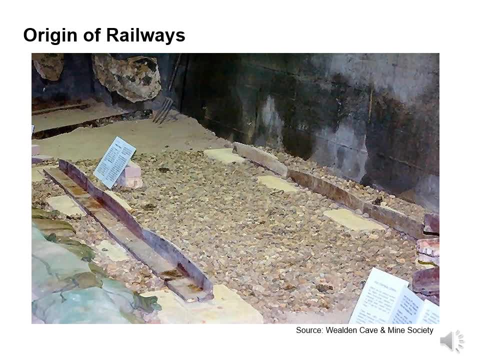 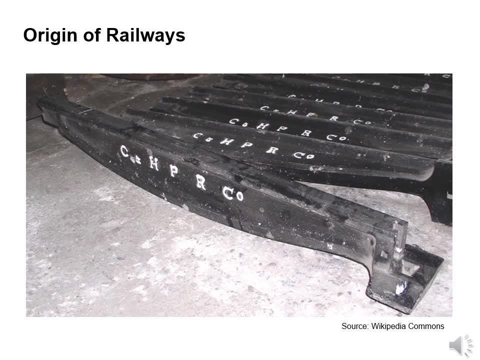 To stop them from spreading outwards. The next important development in iron production Was the hot blasting process Developed by James Nelson, Patented in 1828. Which considerably reduced the amount of coke fuel or charcoal needed to produce pig iron. All these developments in the production of iron eventually led to the replacement of composite wood iron rails. 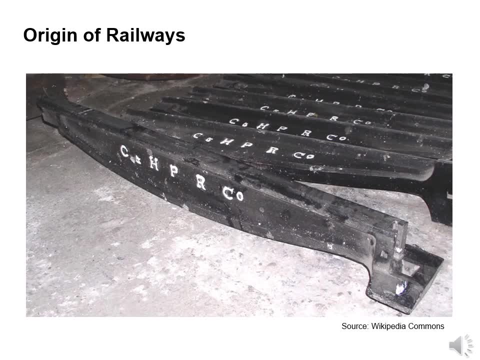 With superior all iron rails. The introduction of the Bessemer process Enabling steel to be made inexpensively, Led to the area of great expansion in the railways That began in the late 1860s. Steel rails lasted several times longer than iron. 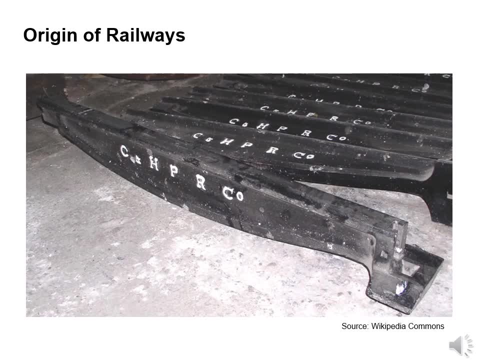 Steel rails made heavier locomotives possible, Allowing for longer trains and improving the productivity of railways. The Bessemer process introduced nitrogen into the steel, Which caused the steel to become brittle with age. The open hearth furnace began to replace the Bessemer process near the end of the 19th century. 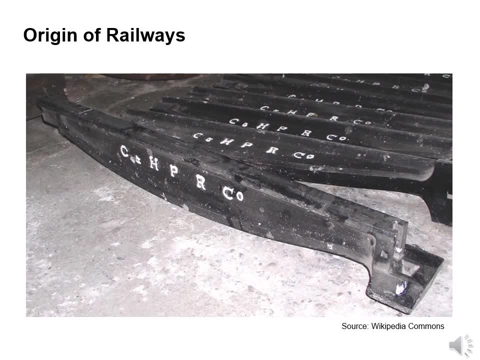 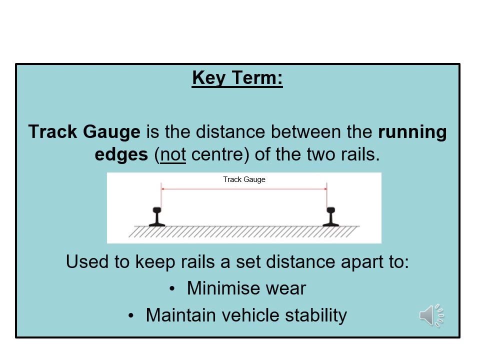 Improving the quality of steel and further reducing costs. Steel completely replaced the use of iron rails, Becoming the standard for all railways. Track gauge is the distance between the running edges, Not the centre of the two rails. It's used to keep the rails a set distance apart. 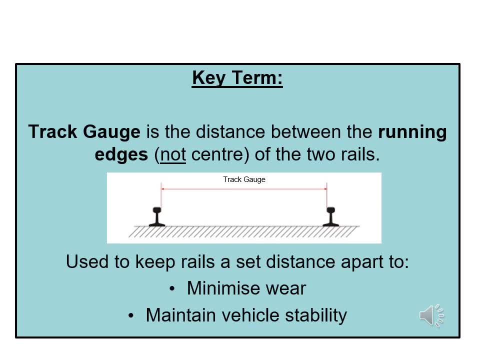 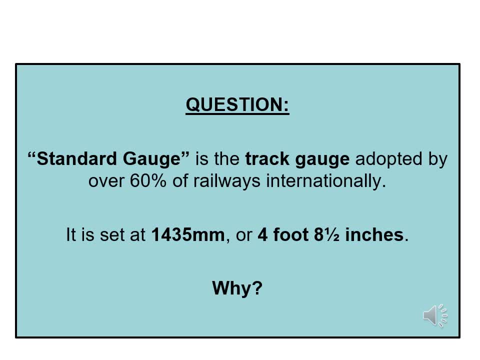 And this minimises wear and maintains the vehicle's stability. Standard gauge is the track gauge adopted by over 60% of the railways in the world. It's set at 1435mm Or, in imperial dimensions, 4 foot 8 and a half inches. 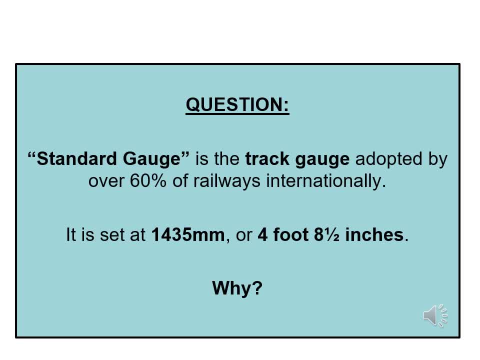 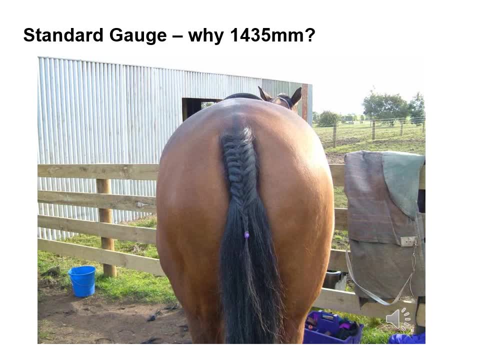 So why did this dimension come about? Well, if you remember, back to earlier on in the lecture, I was explaining that the wagons were often pulled by horses. So this dimension of 1435mm Is quite close to the width of a horse's backside. 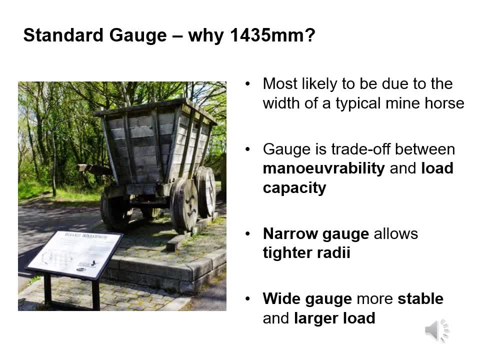 So remember the wooden wagon I showed you earlier on. So these were pulled by horses And this dimension for the gauge Was probably based on a typical mining horse. The gauge is a trade-off between manoeuvrability and load capacity. A narrow gauge allows you to traverse very tight, radius curves. 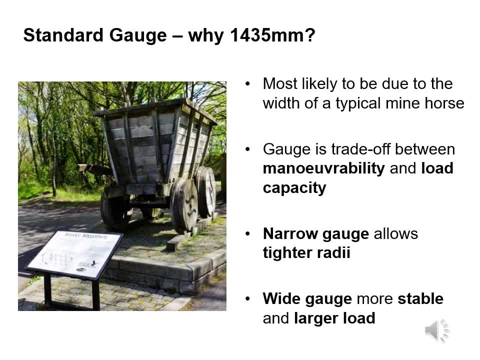 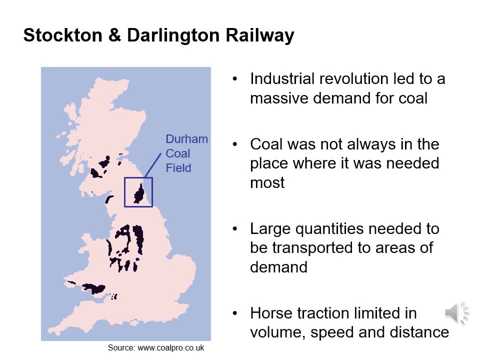 A wide gauge allows for more stable And larger loads. So the industrial revolution led to a massive demand for coal. Remember that the machines That ran the mills Sometimes ran off water, But were often powered by steam. The coal was not always in the place where it was needed the most. 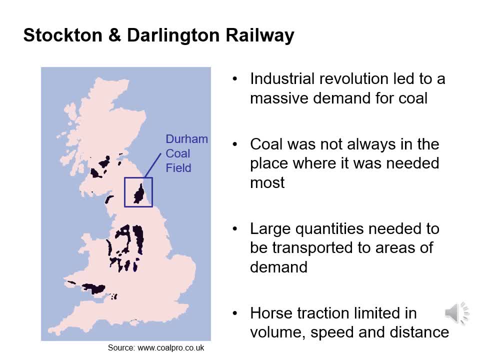 So large quantities of coal had to be transported to areas of demand. Very early on we saw the construction of canals. Canals were a source of navigating The countryside, Eventually into city centres, Where barges could move coal And stone. 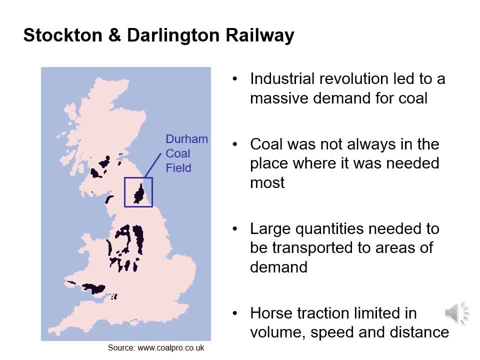 And other materials Into industrial areas. So we had to move lots of this coal, And here you can see an image Showing one of the largest coal fields in the UK, Which is the Durham Coal Field. We were limited by the use of horses. 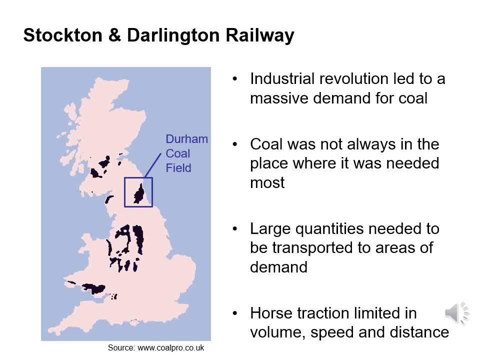 There was only so much they could pull At a certain speed and distance. So we had to move lots of this coal. And here you can see an image Showing the distance. So you can see an Ordnance Survey map Showing the Durham Coal Field. 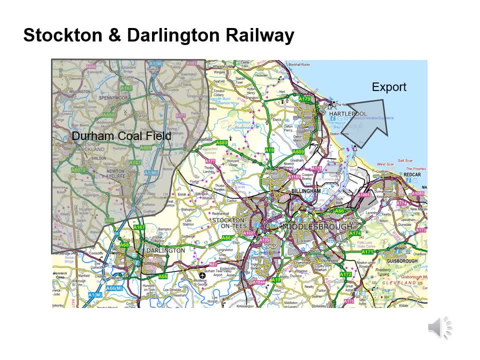 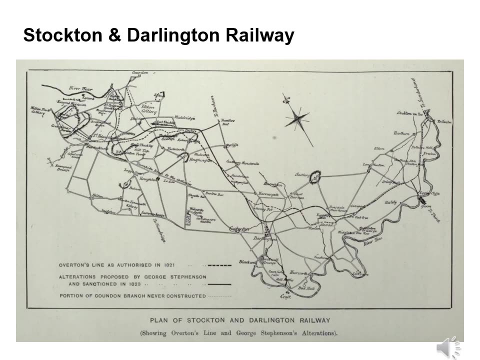 The location of Darlington And Stockton And eventually The harbours which allowed the coal to be exported. The Stockton and Darlington Railway, Which was opened in 1825. Was the world's first permanent steam locomotive hall public railway. 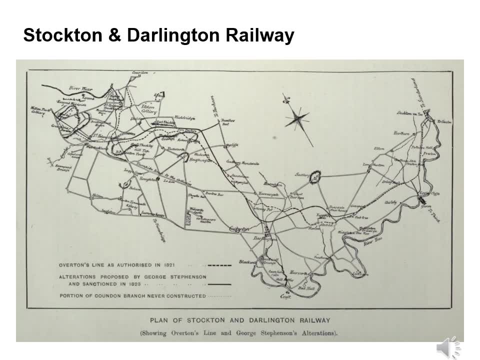 The line, which was 26 miles long, Was initially built to connect inland coal mines to Stockton, Where the coal was to be loaded onto sea going boats. It was also the longest railway at the time, Conceived by a wealthy local wool merchant. 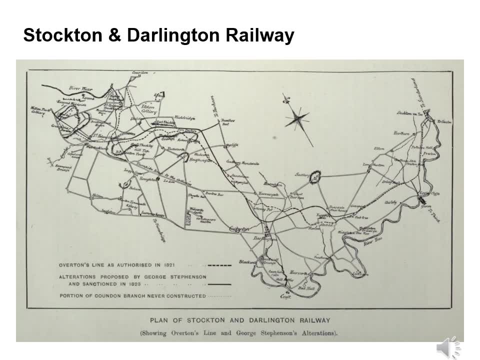 Edward Pease. The Stockton and Darlington Railway was authorised by parliament in 1821. And was initially intended to be an ordinary horse drawn plate way, Which were commonplace at this time in the United Kingdom. However, George Stevenson had been perfecting his engines. 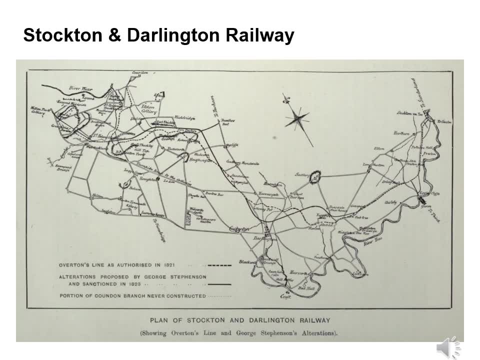 For about seven years He had worked on this project. He persuaded Edward Pease On the day that the act received royal assent, To allow him to re-survey the route And work it At least partly, by steam. Steam traction was expensive at this time. 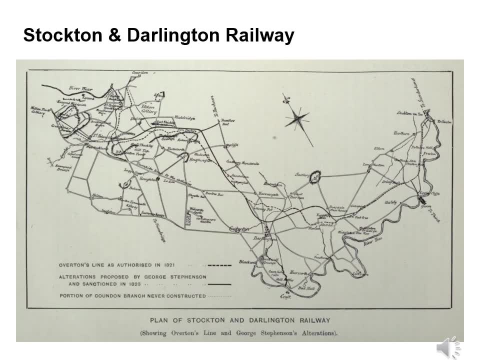 In comparison with horse drawn traffic. But it soon proved that it was a viable and economic solution. Steam locomotives Could haul more wagons, Haul them faster. So on a typical working day The expensive steam engine could haul more coal. 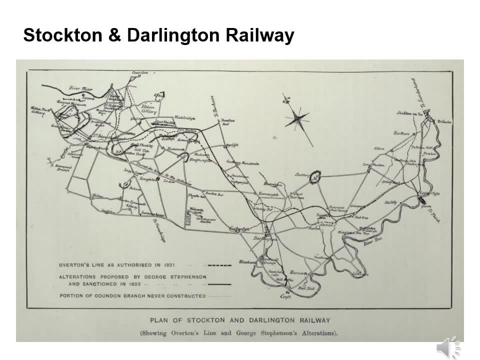 Than the cheaper horse. It soon became apparent That mixing faster steam haul Than slower horse drawn traffic Was slowing the operation down, And so, as steam technology became more reliable, Horse drawn traffic was gradually abandoned. By 1833. The S&DR had become entirely steam operated. 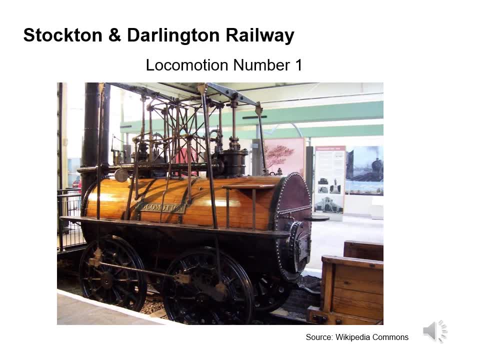 And the steam engine Was the only steam engine That was operated, And it gradually began to resemble a modern railway. The S&DR company became the sole train operator on the line. Parallel double tracks were built For trains travelling in opposite directions. 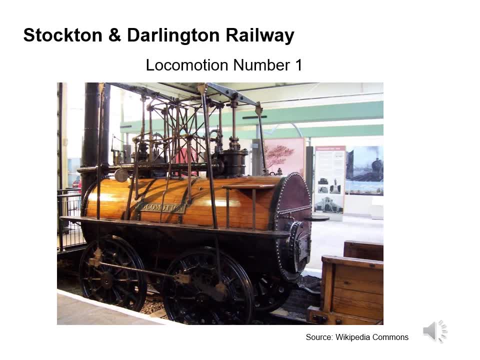 Timetables were established And a crude signalling system was established To prevent collisions. These methods of operation became standard on railways across the world. The S&DR proved To be a huge financial success And paved the way For modern rail transport. 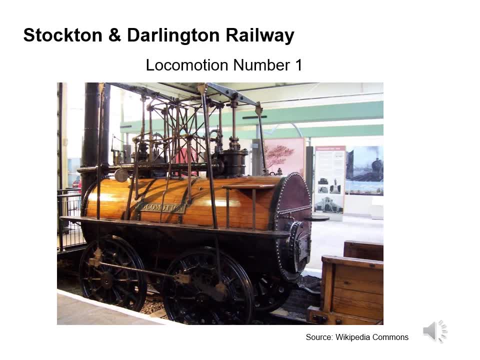 The expertise that Stevenson and his apprentice, Joseph Locke, Gained in railway construction and locomotive building on the S&DR Enabled him, a few years later, To construct the Liverpool and Manchester railway, The first purpose built steam railway, And also his revolutionary 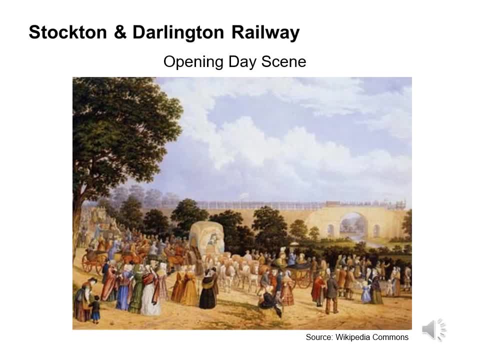 Rocket locomotive. The opening of the S&DR On the 27th of September 1825. Was a great occasion. Not only was it the first public passenger railway in the world, But it was pulled by one of the first steam locomotives. 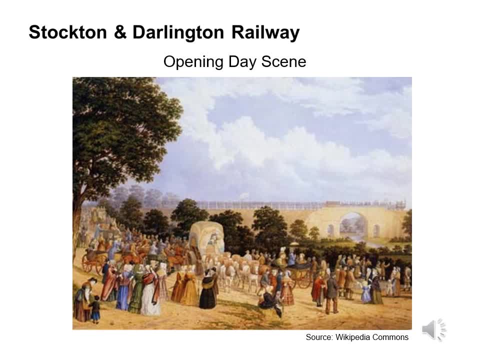 Most people had never seen anything like this before, And 40,000 people turned out to witness it In. this painting By John Dobbin Shows locomotion, one Pulling wagons full of coal flour And, for the first time, people. 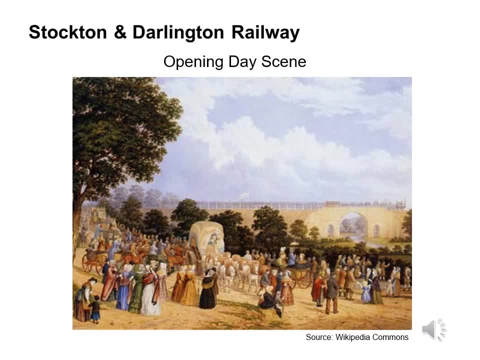 Across Skern Bridge, One of the world's first railway bridges. Dobbin was born in Darlington And would have been about 10 years old When the railway opened. He painted this 50 years later From sketches made by his father. 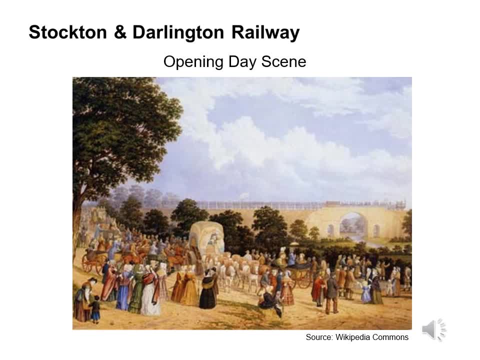 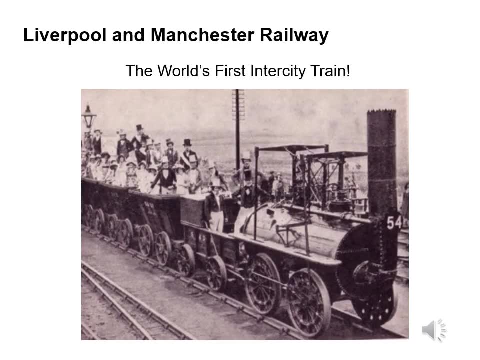 And possibly from his own memories of the day. This is his most famous painting And an important record Of this world famous occasion. The Liverpool Manchester railway Was the world's first intercity passenger railway In which all the trains were timetabled. 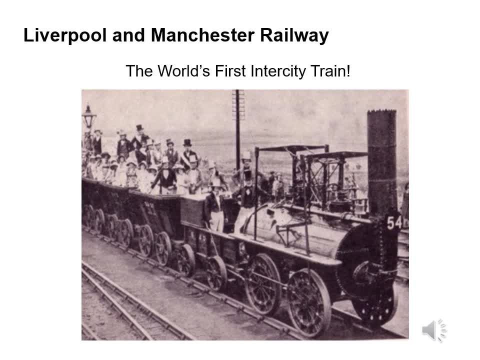 And were hauled for most of the distance Solely by steam locomotives. The line opened on the 15th of September 1830.. The line was primarily built To provide fast and cheap transport Of raw materials and finished goods. 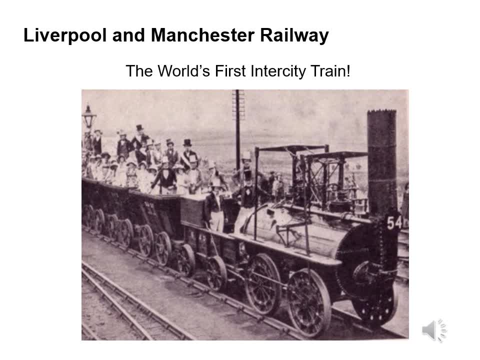 Between the port of Liverpool And the mills in Manchester And surrounding towns of East Lancashire. Huge tonnages of textile raw material Were imported through Liverpool And carried to the textile mills Near the Pennines, Where water and then steam power. 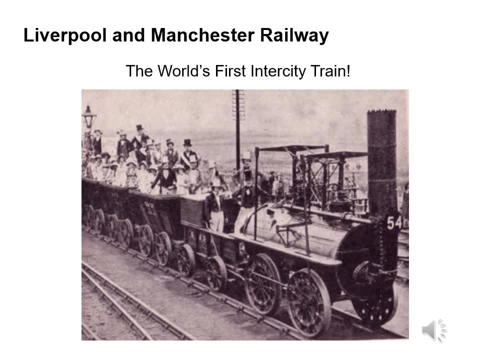 Enabled the production of the finished cloth. The existing means of water transport, The Mersey and Irville navigation And the Bridgewater canal, Which dated from the previous century, Were felt to be making excessive profits From the existing trade And throttling the growth of Manchester. 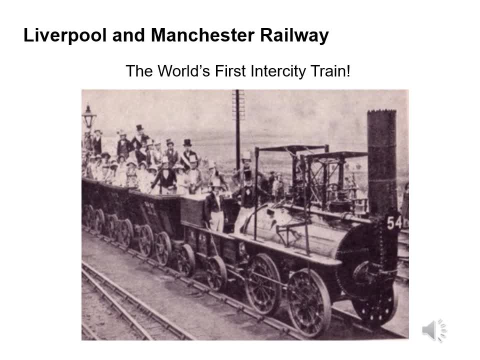 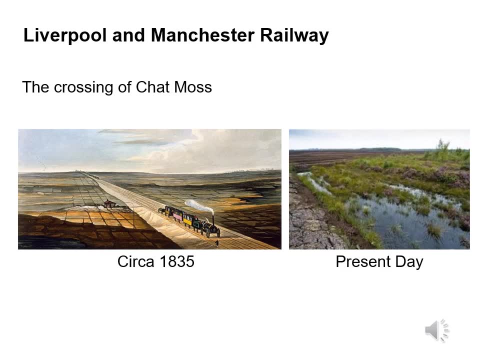 And other towns. There was support for the railway From the cities at either end, But opposition from the land owners Over whose land the railway was proposed to pass. The 35 miles of line Was a remarkable engineering achievement For its time. 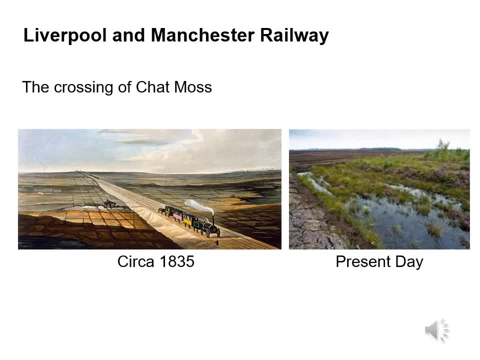 Beginning With the 2057 metre Whopping tunnel Beneath Liverpool. Following this was a two miles long cutting Up to 70 foot deep, Or 21.3 metres deep, Through rock at Olive Mount And a nine arch viaduct. 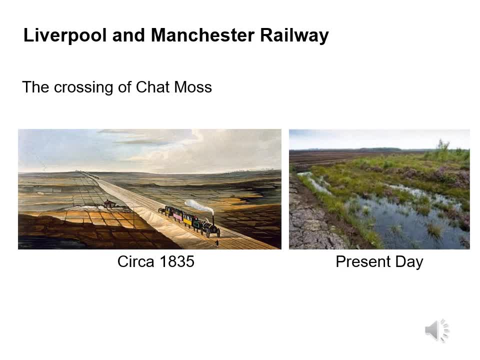 Each arch A 15.2 metres span Over the Sankey Brook Valley And it was around 21.3 metres high. Not least was the famous 4.75 miles Crossing of Chat Moss, Having found it impossible. 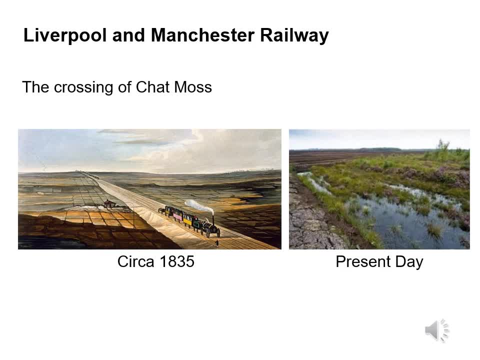 To drain the bog, Stevenson began constructing A large number of wooden And heather hurdles, Which were sunk into the bog Using stones and earth Until they could provide a solid foundation. It was reported that at one point, Tipping went on solidly for weeks. 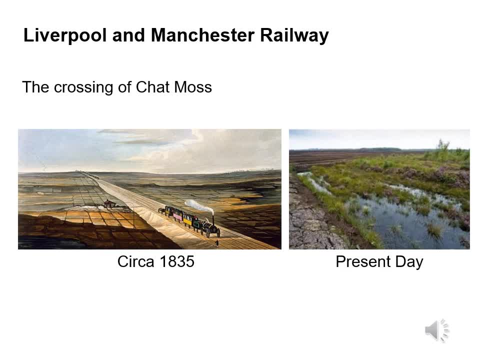 Until such a foundation had been created. This was also the technique they used. Across Rannoch Moor In the Highlands of Scotland At the time of the loss Floats on the hurdles That Stevenson's men laid, And if one stands near the line side. 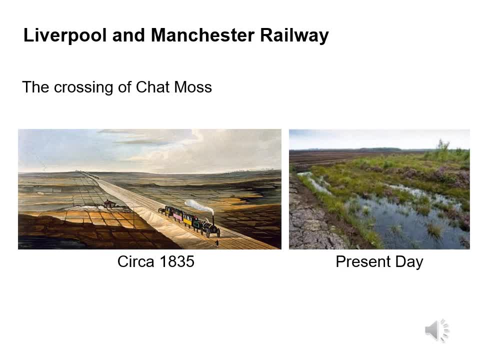 One can feel the ground move As the train passes. It's worthy to note That the line now supports locomotives Twenty times the weight of the rocket Which hauled the first experimental train Over the moss In January 1830.. 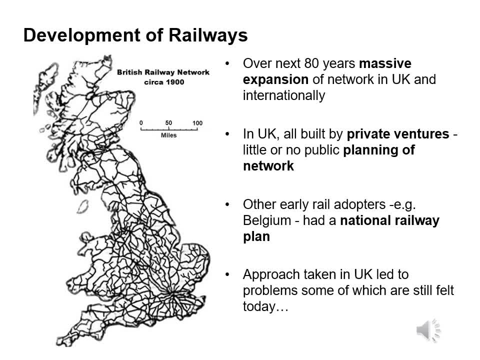 Over the next 80 years There was massive expansion of the network. It was all built by private ventures With little or no public planning of the network. Other early rail adopters- EG Belgium, Had a national railway plan- The approach taken in the UK. 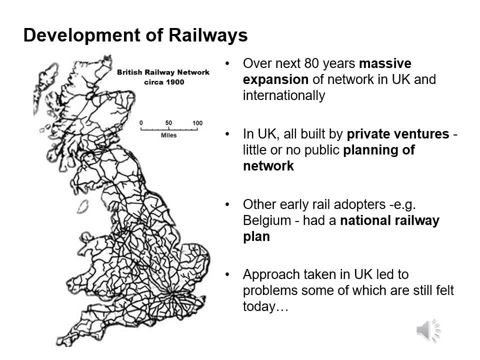 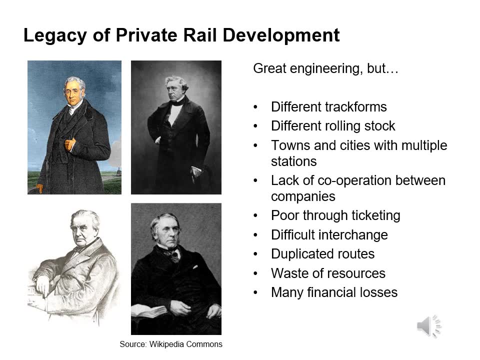 Led to problems, Some of which are still felt today, And you can see from the image here on the left How extensive that network was In around 1900.. So what were the legacies of this private venture, Private rail development? 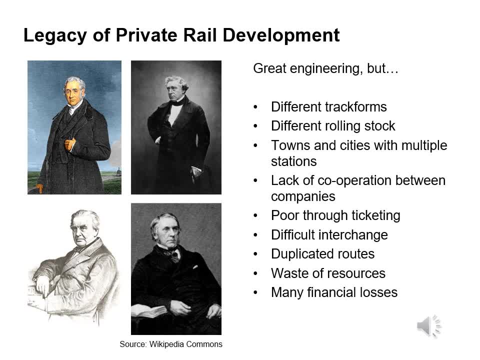 Well, we had some of the greatest civil engineers of our time On the projects: From top left, George Stevenson, Then top right, Robert Stevenson, Bottom left, Charles Vignole And then bottom right Joseph Locke. Some great civil engineers. 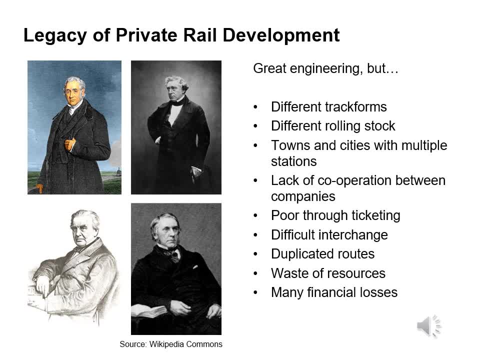 And some great engineering, But there were problems With different track forms, Different rolling stock, Towns and cities with multiple stations, Lack of cooperation between companies, Poor through ticketing, Difficult interchange, Duplicated routes, Waste of resources And projects which went wrong. 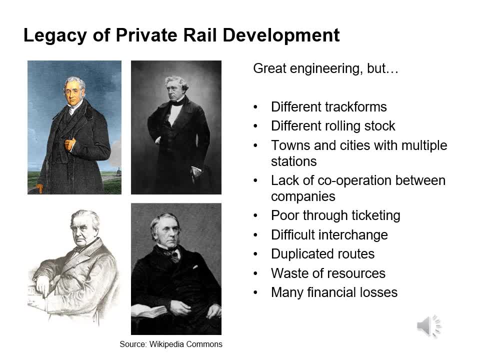 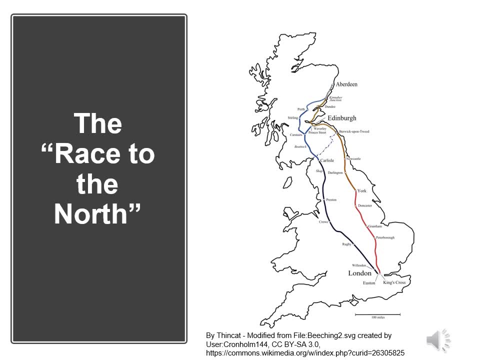 And resulted in huge financial loss. Some of these problems still exist today. The Race to the North Was the name given by the press To occasions Two summers of the late 19th century When British passenger trains belonging to two different companies 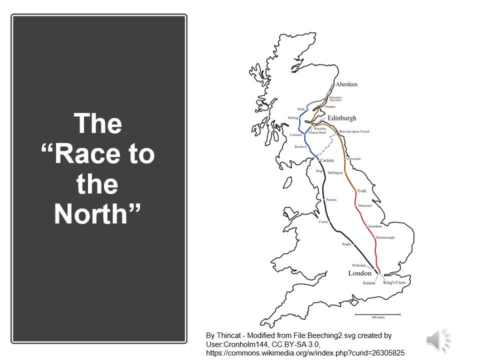 Would literally race each other From London to Edinburgh Over the two principal rail routes Connecting the English capital City to Scotland: The West Coast Main Line, Which runs from London-Houston Via Crewe and Carlisle, And the East Coast Main Line. 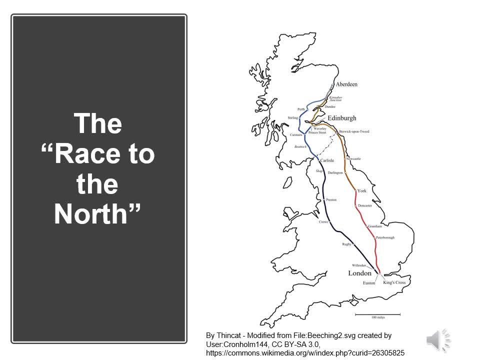 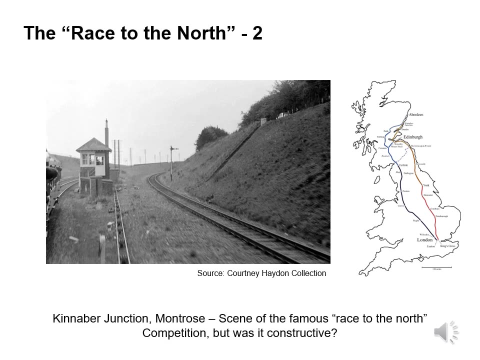 Which runs from King's Cross Via York and Newcastle. The races were never official And publicly the companies denied That what happened was racing at all In 1895.. A second race broke out, But this time with the added excitement. 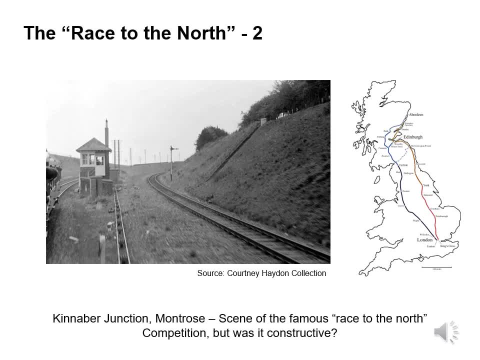 Of arriving at the same station in Aberdeen. Indeed, after some 500 miles from London, The two routes converged To being in sight of each other Just before Canaver Junction, From where there was a single track to Aberdeen. So consider Manchester City Centre. 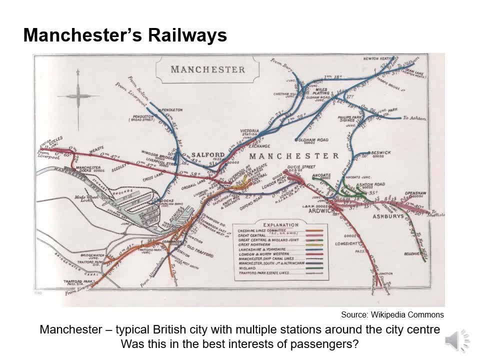 It has four main railway stations- Piccadilly, Victoria, Oxford Road And Deansgate- Which all form part of the Manchester Station Group, And the reason why We have four stations spread across the city Rather than one big central station. 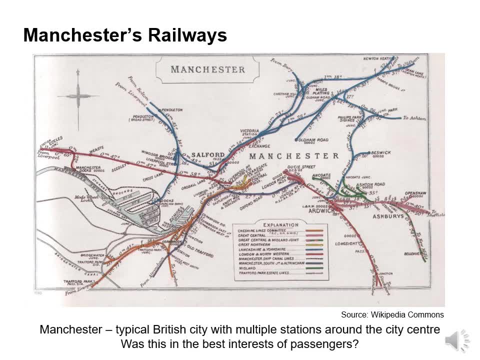 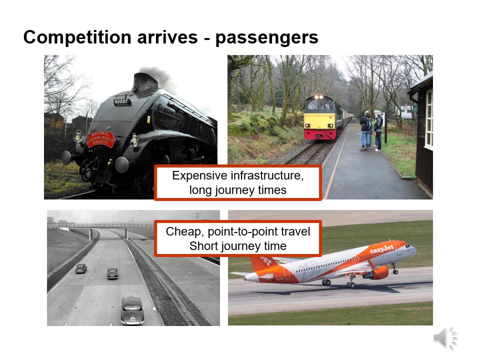 Is because of the competition With the early development of railways. Now my question is: Is this in the best interests of passengers? So, when competition arises, What do passengers want? Do they want expensive infrastructure And short journey times, Or do they want cheap, point to point travel? 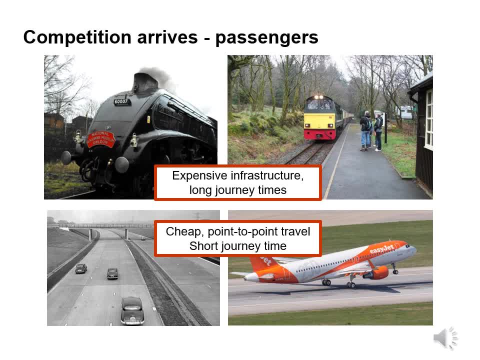 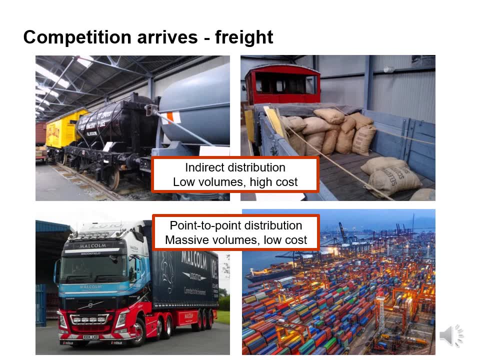 And short journey times. In terms of freight, Well, the railways provided indirect distribution. They could only carry low volumes And they were pretty costly. But then we see Point to point distribution Provided by trucks, Massive volumes from shipping And again low costs. 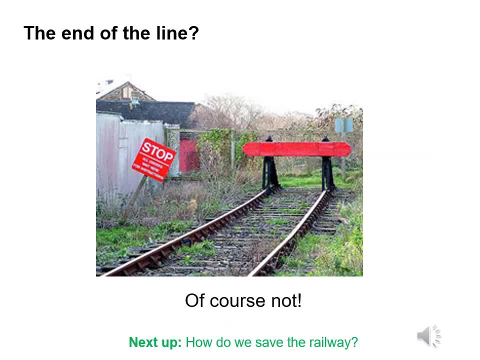 And the fact that They can't even operate When they can't even drive, When they can't even drive Any doing anything. They have lots of workers And it's very expensive, Unfortunately, But they can't really do nothing. 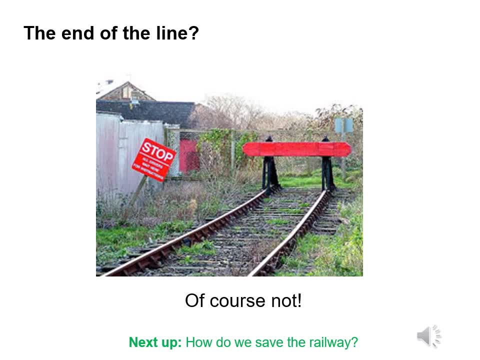 So they're really just Their own real time job, And that's what makes them small And they can do anything. So they can do anything they want, Everything they want, And you can throw a car In the car. You can throw a car. 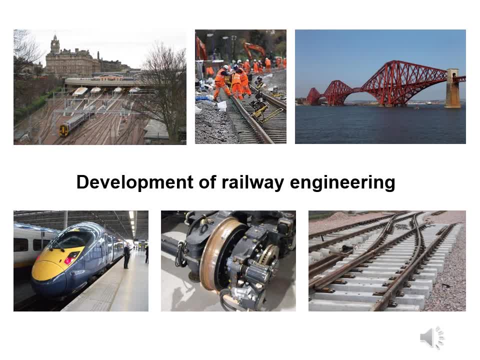 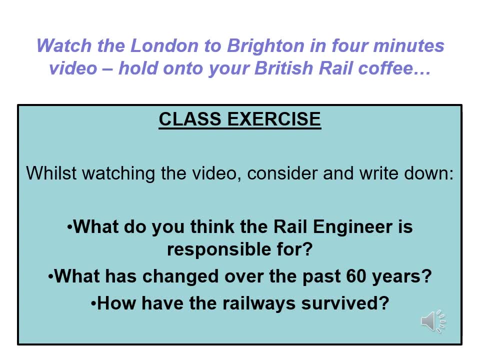 Anything you want, They can cool it down, And then they can Move it around, And then they can do anything they want And they'll fly And they won't. That's where my point is is pause the video here and watch the london to brighton in four minutes video. 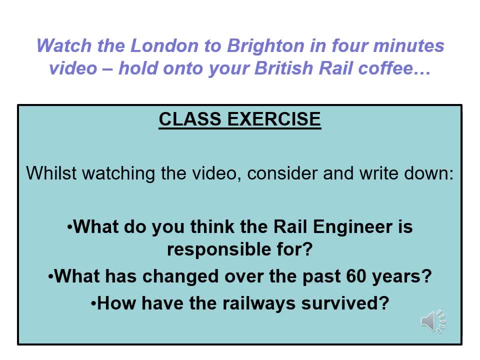 that's on the virtual learning environment. that's middle. make sure you hold on your british rail coffee, because it's quite a ride. and i want you to think about the three questions below. so what do you think the rail engineer is responsible for? what has changed over the past 60 years and how have the railways survived? 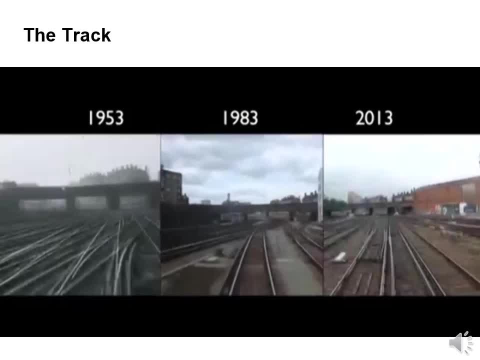 so the figure here shows the same location in 1953, in 1983 and then in 2013.. in 1953, the track was much more complex and extensive than in 83 in 2013.. at the time, rail in the uk and much of the world was becoming inefficient and costly and had not kept up with. 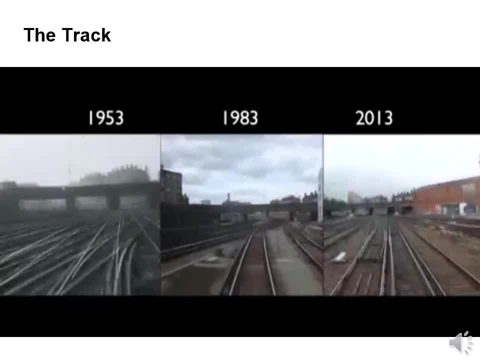 changing transport habits. by the 1980s, rationalization had occurred throughout the beaching cuts in the uk which happened in the late 60s, and railway was in decline. in the current day, patronage growing and station approaches are optimized for maximum capacity with simple layouts. 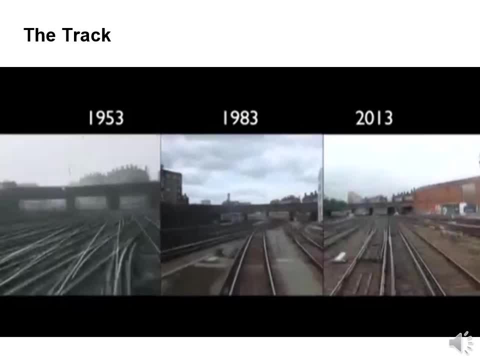 the rail engineer responsible for the design of these layouts and components. design includes formation sleepers, fasteners, rails, switches and crossings. what you probably couldn't see was that the sleepers back in 1953 were predominantly wooden and the track was made out of two pieces of. 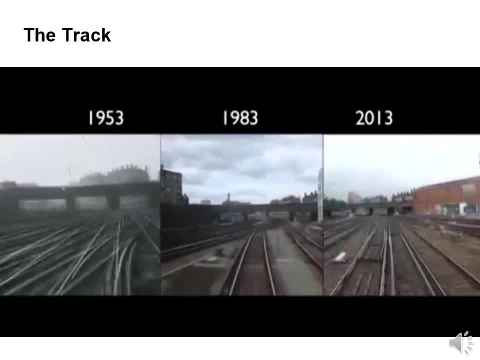 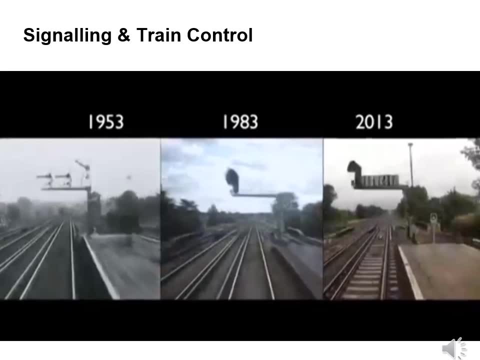 much more likely to be jointed rather than continuously welded rail. so now we're going to look at the signaling and train control systems. in 1953, signals on this line were operated by a semaphore system. this was a system of mechanical levers and metal wires. the lines were broken up into hundreds of blocks and 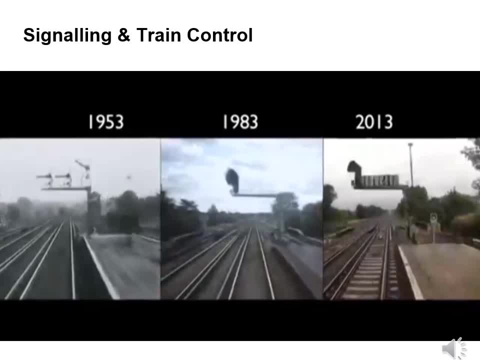 these were controlled by dozens of signal people or signal persons in local signal boxes along the route. by 1983, electronic signals were installed in this line, but not the semaphores are still widely used even to this day. in 1983, control was by a remote signaling center rather than signal boxes. in 2013, 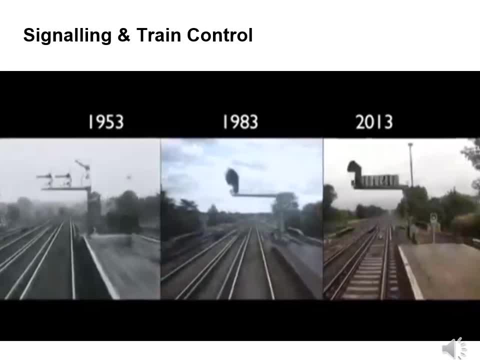 the signals were much the same, but control was further centralized for greater efficiency. it may not be clear on this slide, but some new technology was introduced. for example, in 2013 we'd see LED lights in the signals. also in this slide you can see AWS automatic warning system, TPWS- train protection warning system- or 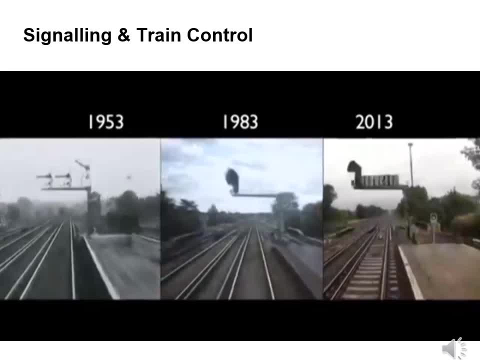 automatic train protection units and these were installed to act in case of driver error. so if the driver passed a signal at danger, ie red, the train would automatically apply its brakes. we'll go into more detail about these systems further on. in the module 1953 the only interface between the outside world and the train was the 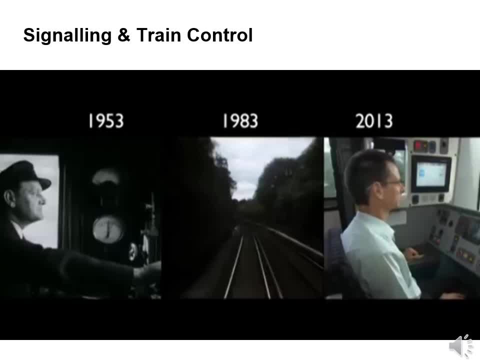 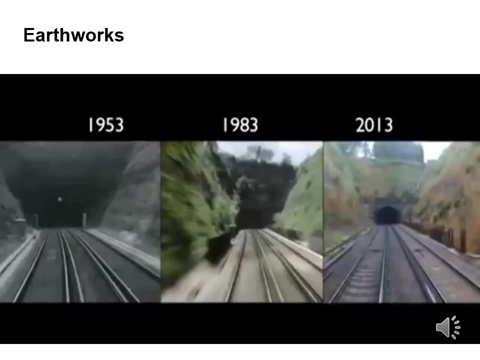 drivers eyes and the signals. in 2013, trackside communication systems and onboard safety systems mean that some systems have no signals and some even have no drivers, for example, the Docklands light railways system. so here you'll note that the tunnel remains the same. so this was Victorian infrastructure that is still in use today. 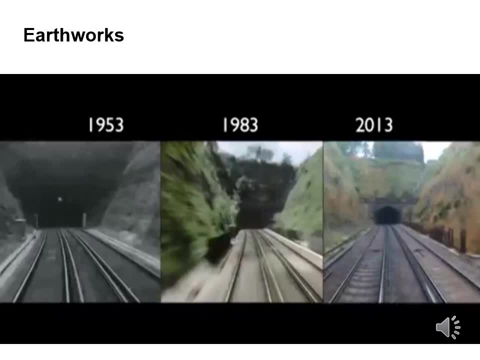 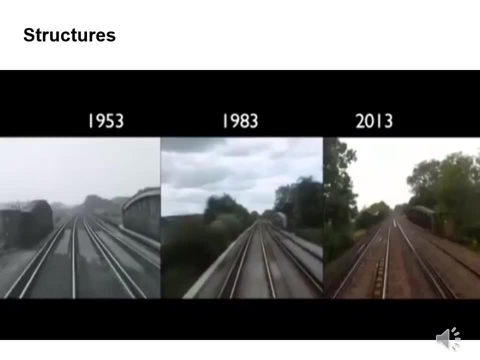 so this was Victorian infrastructure that is still in use today, in operation today. So in this slide you'll note that the bridge in 1953 is the same bridge in 1983 and the same bridge in 2013.. Again, we see historical. 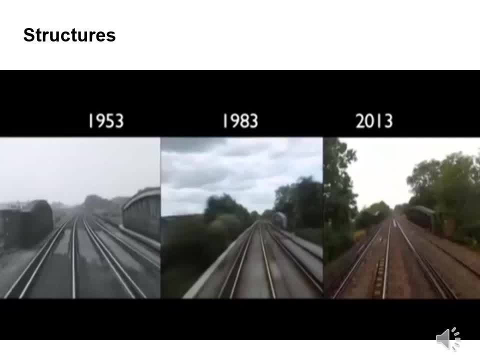 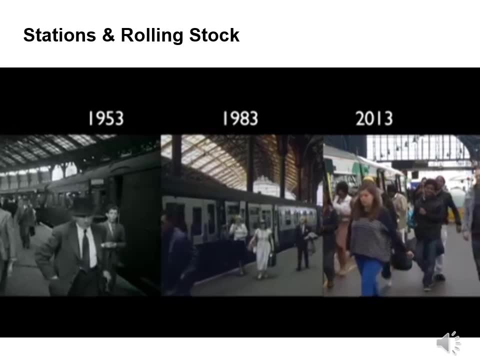 infrastructure still in operational use in present day, So it is a rolling stock. Much of the rolling stock in the 1950s consisted of a locomotive hauling a passenger train, which is made up of carriages. When that train pulled into a station, what happened was the locomotive would end up at the buffers. Another 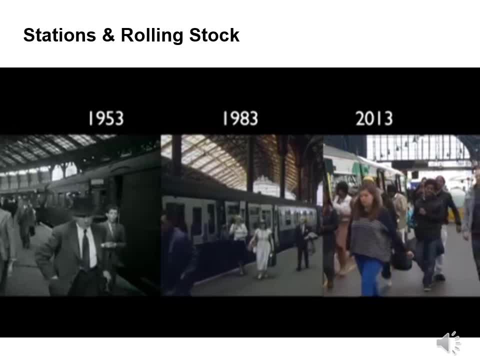 locomotive would then have to come in and connect to the the rear of the passenger train. Obviously they decoupled the original locomotive. The new locomotive would then pull the train away with the new set of passengers. That would then release the original locomotive. 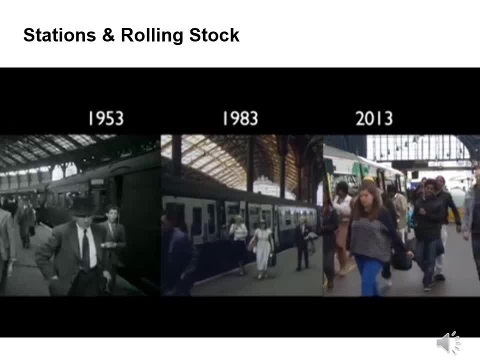 and this required changeover times and also station staff to go down and decouple the locomotive from the train. This was also timely and expensive as well. So modern rolling stock is generally formed by multiple units with cabs- driver cabs- at both ends. Another thing that's changed is in the 1990s. 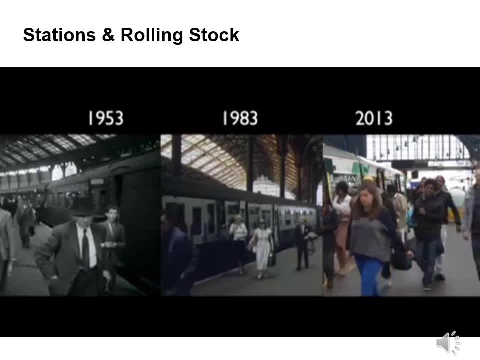 central door locking was fitted on passenger carriages and this was to replace a lot of the old side doors. It was a slam door stock that was phased out due to safety concerns. That was stock which could allow the passenger to open the door whilst the train was still. 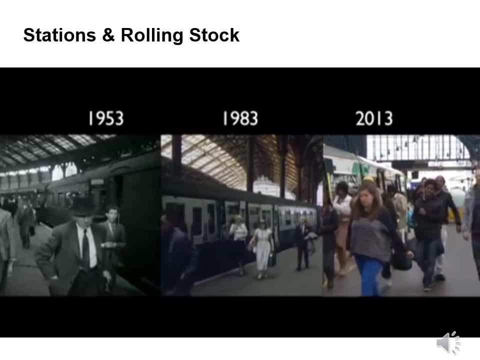 moving. So trains have become increasingly faster- not so much top speed, but more acceleration- and electric units are now more common throughout the country. In terms of the stations, the changes are a little more subtle. The expectations of stations by rail companies and passengers are more of a destination with lots of retail. 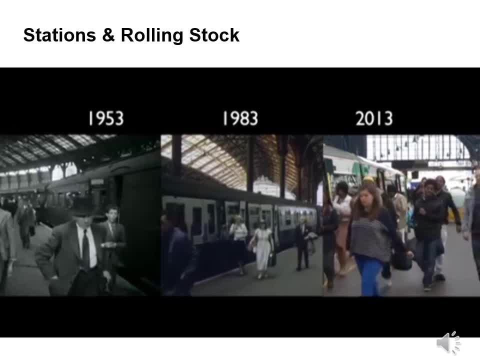 space Facilities such as food outlets, cash machines, even supermarkets are now expected. So passenger numbers are on an increase. overcrowding at stations is often an issue, and they need to maximise the efficiency through which passengers can move through the station. So we see things now like automatic barriers, ticket machines, and this all adds to the 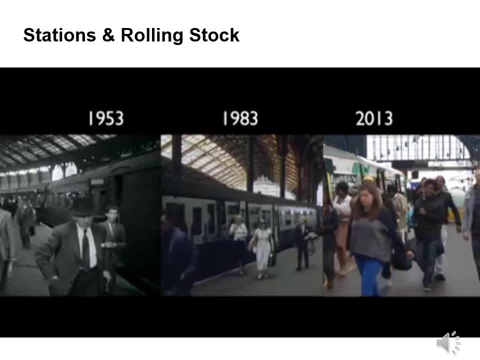 efficiency of the passenger experience. Accessibility is an issue in some of the old Victorian stations. The new KFW stations, as you'll see here, are set up for use by the DuPont сюין are another experimental education system based on authoritative scientific research. As you can guess, you could use them as a. 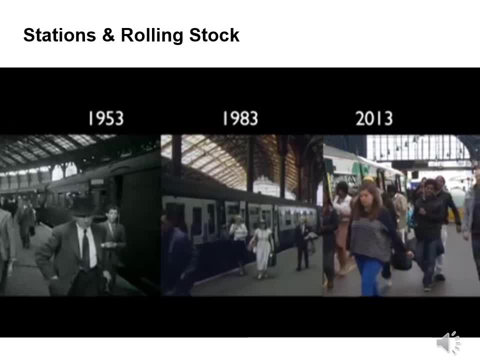 demonstration: The UCL train can now stay in our vuhtalous conditions all day. This isリズ distortion period, so we've been able to experience the value of ook allem on long before we mine. and power on the c broaderah eyeball. 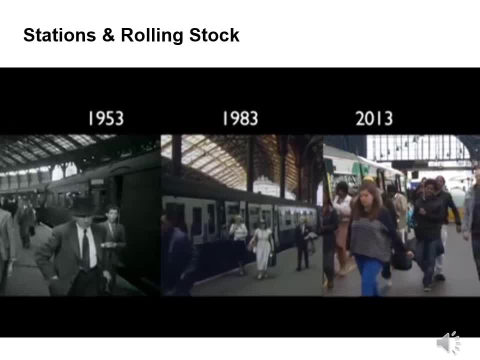 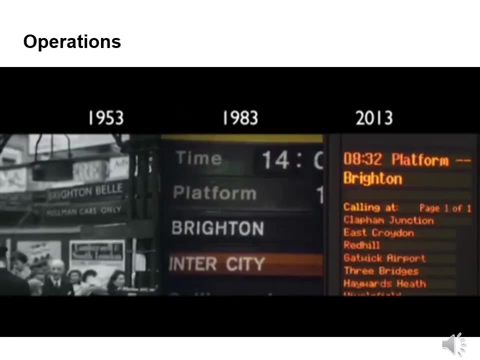 lots of extensions to platforms and lots of refurbishment projects where Victorian stations have seen significant alterations and improvements, and the most recent one in Edinburgh was Waverley station. In terms of operations, railways in the UK are now carrying more passengers with less track. Trains are running more frequently than ever In 1953. 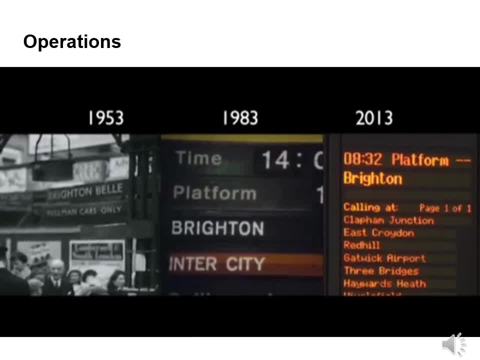 there were six trains per hour from London on the Brighton line. There are now 19.. London to Brighton back then took 60 minutes. now it takes 52 minutes. Unlike private road transport, trains run to a timetable and passenger expectations are high. Trains cannot take alternative routes. therefore, 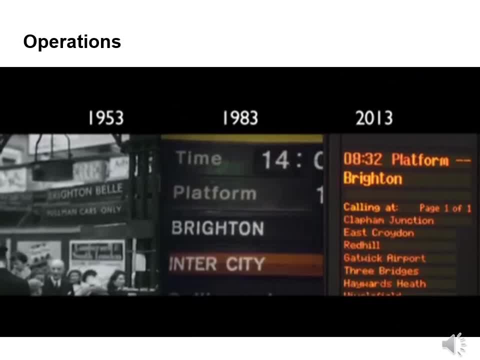 the risk of disruption by unexpected events is high. Operations involve timetable planning, staff rostering and equipment scheduling. It involves several factors: a cost benefit analysis, defining stopping patterns. route constraints- eg signaling. rolling stock capability- eg acceleration, deceleration. and capacity and reliability considerations- eg engineering works on the track. 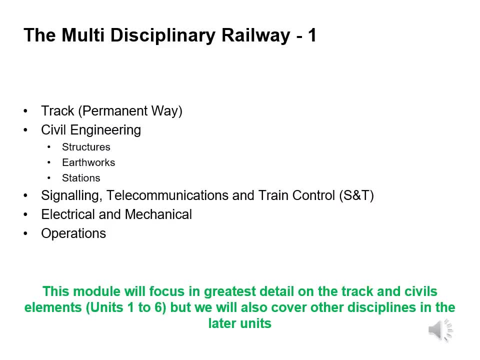 So the railways multidisciplinary. Some of the disciplines we see in the rail sector include track permanent way engineers, commonly known as p-way engineers, civil engineers, which design structures, earthworks and station buildings. We also have those concerning themselves with signaling, telecommunications and train control. 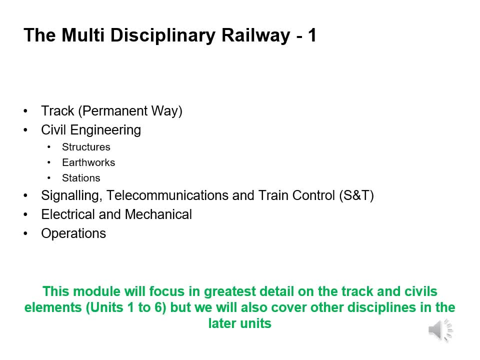 known as S&T. We have electrical and mechanical engineers and we also have those who specialise in the operations of the railway. So this module will focus in greatest detail on the track and civil's elements. We're going to see that in units one to six, but we'll also cover other disciplines. 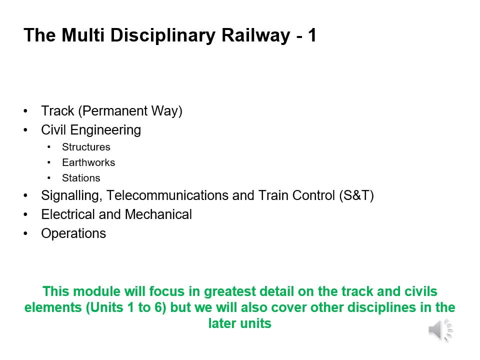 in the later units. So this is our另ę. It's going to be detailed supper on a platinum level. that's a dinner for those of you who are new to the class, So it's going to be a lot of class this time. 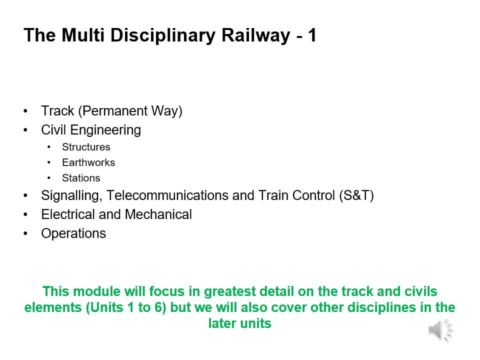 That's a lot of customers, there's a lot of their race and it's going to be a lot of fun and I'm going to show you all of the disciplines that I have in the test track. It's going to be a lot of fun, but it's really going to be a lot of fun, so it's really going. 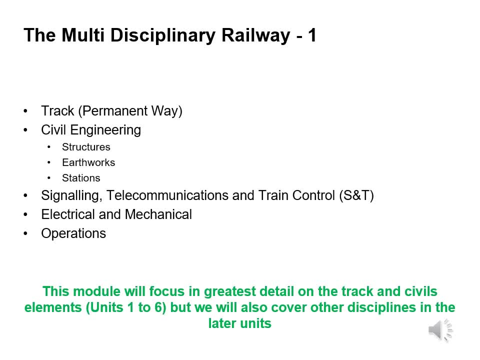 to be a lot of fun. You guys have no idea that there's so many things that I've been working on this week and I'm going to be a lot of work on this week, but this week's test track is really going to be a lot of fun. 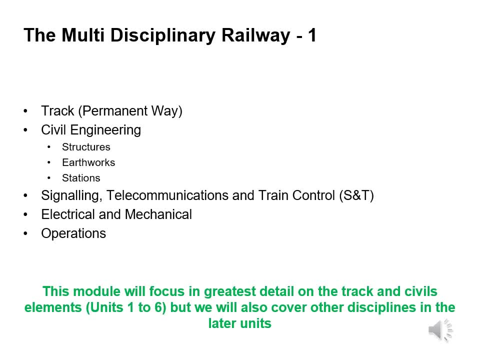 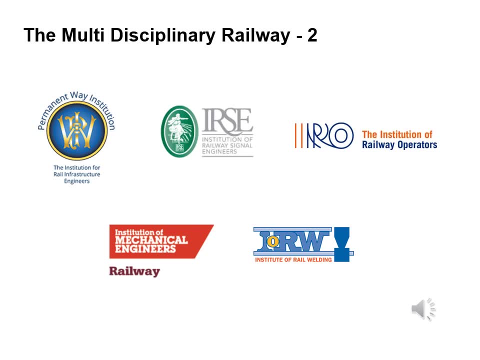 So, as we have a multidisciplinary railway, we have a range of institutions which allow railway engineers to gain professional accreditation, the first of which is the Permanent Way Institution. We also have the Institution of Railway Signal Engineers, the Institution of Railway Operators. 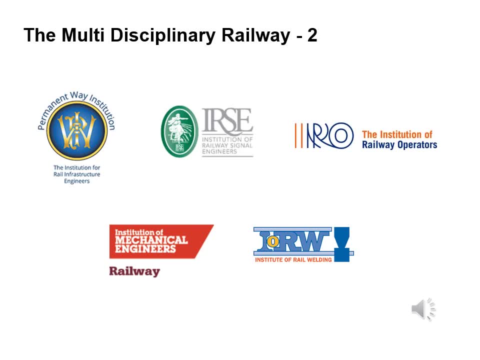 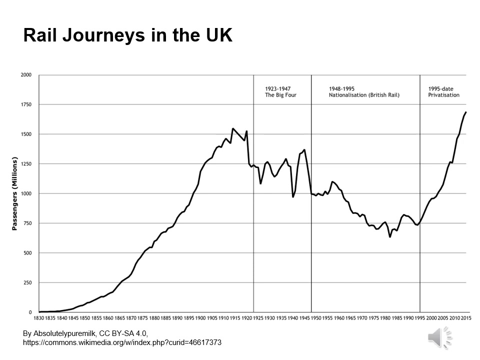 the Institution of Mechanical Engineers and the Institution of Railway Welding. This graph shows the Permanent Way of Railway. This graph shows the Permanent Way of Railway. This graph shows the Permanent Way of Railway. This graph shows the number of passengers, and millions, that were using the UK Rail network from a period of 1830 to 2015.. 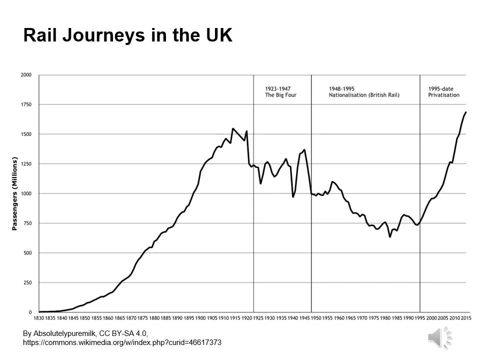 So I want you to spend some time looking at this chart and think about where you see a change in the number of passengers. what happened at that point in time? So, for example, did the car suddenly be introduced? Was there a world war? 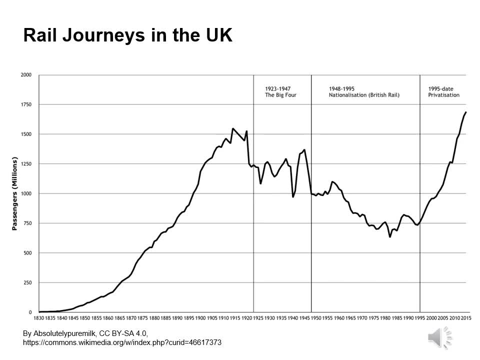 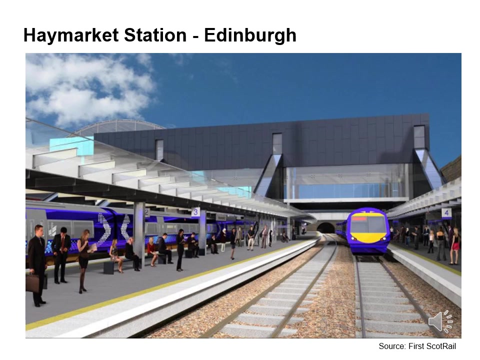 Or, sadly, was there a series of railway accidents. In 2013, Haymarket station saw a 25 million pound redevelopment project. Prior to this, the station had some serious problems, in particular, the volume of passengers that could move through the station at peak times. 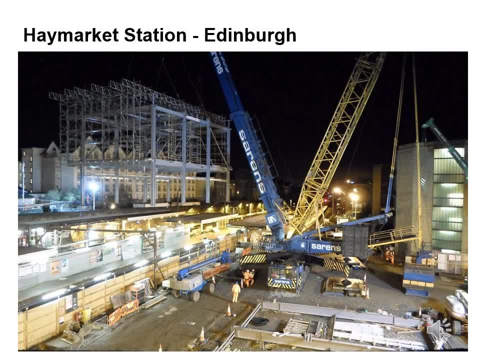 So you can see an image of the main contractor lifting the grey steel superstructure into position. This was undertaken in the evening during an engineering possession. The contractor pre-assembled the steel on site and then lifted it into position once complete, and this minimized the disruption to passengers. 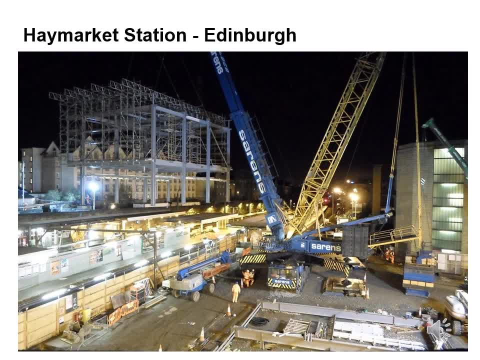 during the construction of the station. During this project, the station had to remain operational- an extremely challenging project to build, basically a new station building whilst the station remained operational and ensuring the safety of the passengers. Here you can see an architect's impression of the finished ticket hall. 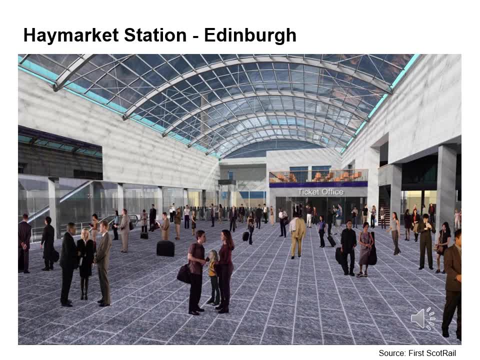 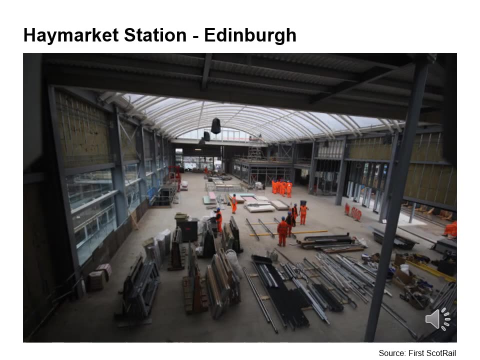 A bright open space, a new ticket office, new destination boards and a significant improvement to the number of entrances and exits to the building. Here you can see the ticket hall taking shape. Note that all the staff on site are all wearing orange high visibility clothes. 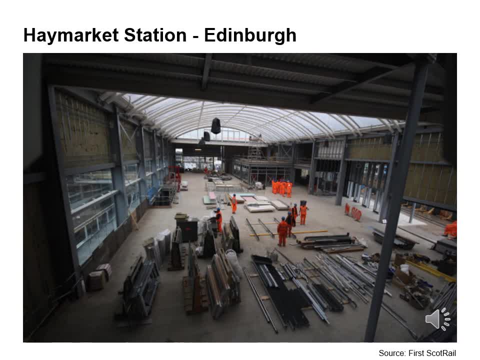 That's because they're working in the rail sector. You can see the roof structure is complete, the site's dry, but also note how carefully organized all the materials and components are on the site. A very clean and well-organized site. a credit to the main contractor. 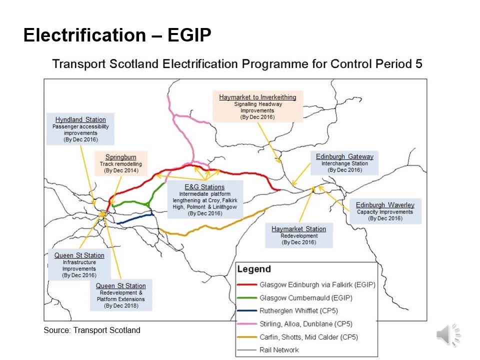 The Edinburgh and Glasgow improvement program allowed the construction of overhead line electrification, known as OLE, and the subsequent introduction of electric multiple units For services on the Edinburgh to Glasgow line. piling works were required for installation of support masts and gantries. The project included all the civils work track improvements, S&C. 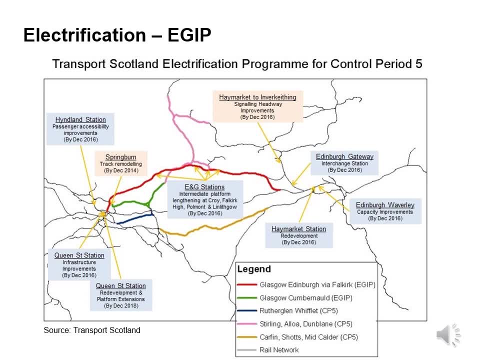 upgrades, junction redesign, signalling and telecoms infrastructure to upgrade the route in parallel with the electrification works. The project enables faster, modern, cleaner and quieter trains to run in these lines. The project required investment to clear bridges on the route and ensure that electrification lines could be installed safely underneath structures. 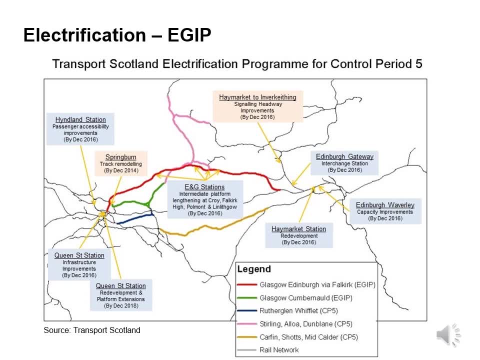 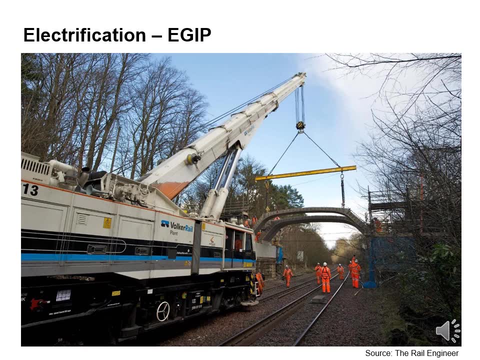 The line was eventually energized for use in September 2017.. The civils work included the design and construction of new bridges to ensure the overhead clearance for the new overhead line. electrification- Here you can see a Volcker Rail rail crane lifting precast concrete bridge sections into place. 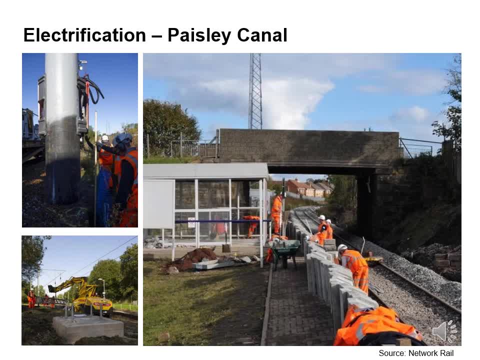 So you can see up left the piling works for the installation of the foundations for the overhead line electrification masts. Bottom left you can see a reinforced concrete pad foundation with holding down bolts ready to receive the base plates. On the right. what's happening here is they've lowered the track rather than altering the bridge. 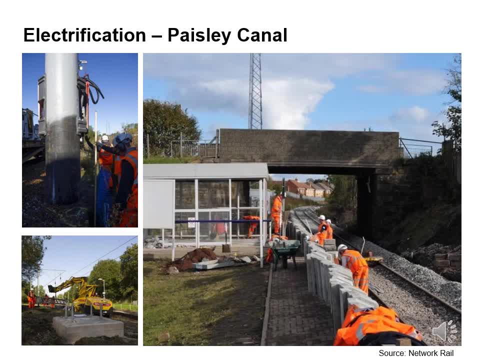 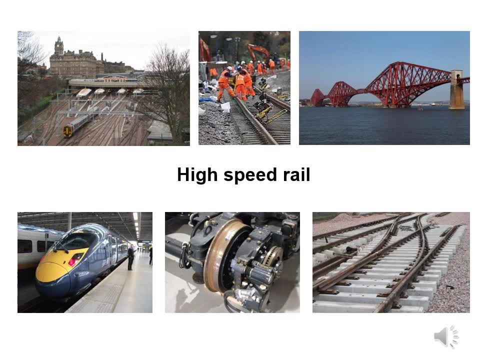 and as they've lowered the track, they're then having to adjust the platform level accordingly. So in the last part of this lecture we're going to examine the principle of high-speed rail. We're going to consider the ongoing development of such rail technology in the UK. 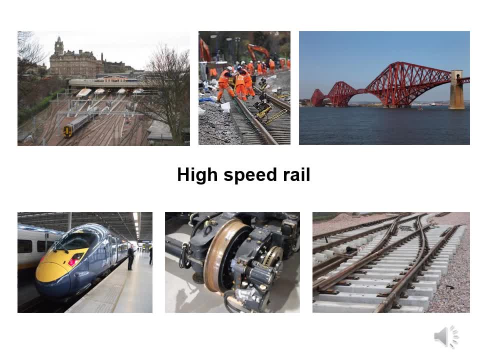 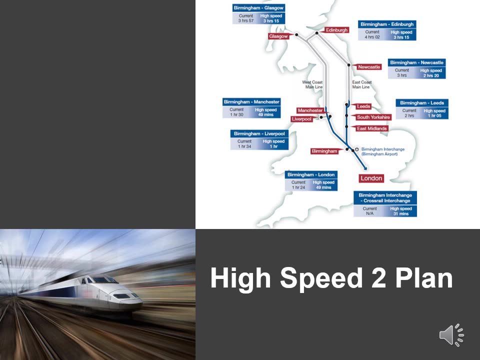 and internationally. This is a specialist subject in its own right. The specific technical details of high-speed rail are beyond the scope of this lecture. High-speed 2 is a new high-speed railway line that's been proposed to link the north of the UK with London. It is aimed to improve the rail capacity of the UK and connect the north. 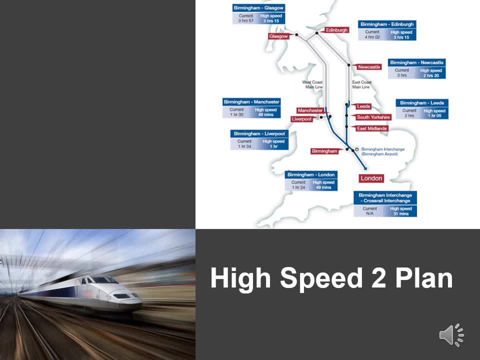 and the midlands of the UK to London. Its aims Are to help rebalance the economy and remove the focus from just London. The three main benefits of HS2 are the capacity to free up space on the existing network for commuters and freight trains. 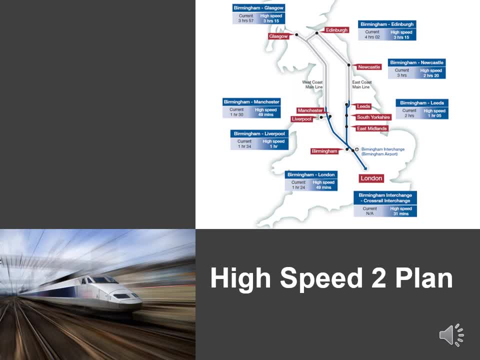 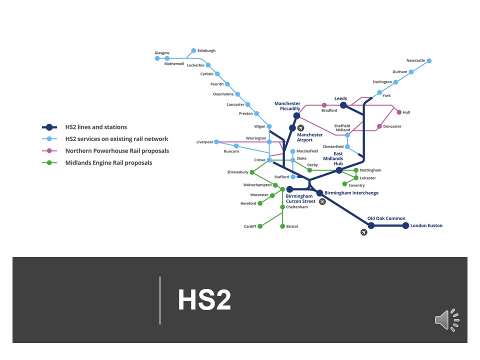 To provide better connectivity, better links between major cities, to level up the country, as Boris says, And to reduce carbon emissions, to emit less pollution, considering if passengers are using cars or planes to travel the length and breadth of the country. This slide shows a map of the new HS2 lines and how these will connect to the existing network. 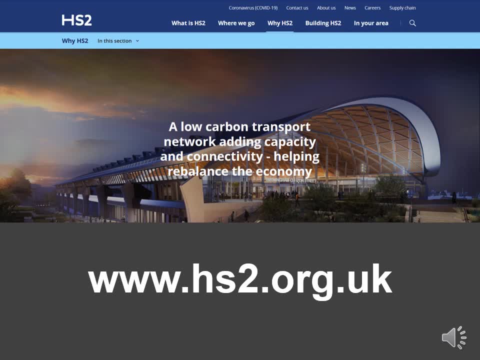 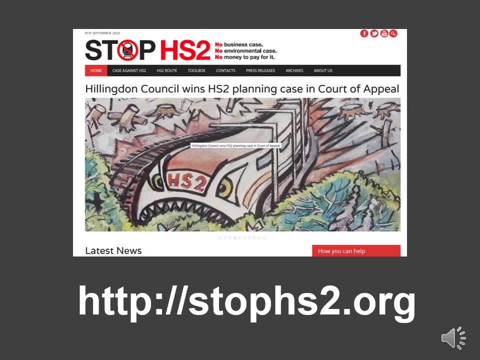 The HS2 project has a dedicated website to keep the public informed of the progress of the project. Have a look at the website and have a look at some of the recent updates. As before, we have a normal elements to consider before you move to the new HS2 line for categories. 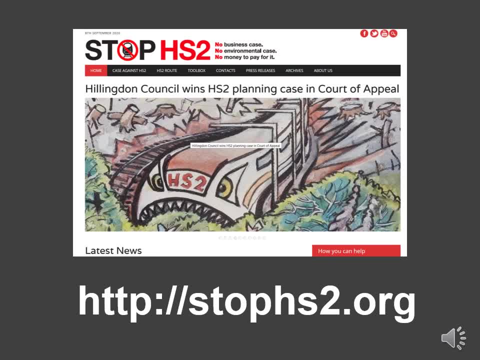 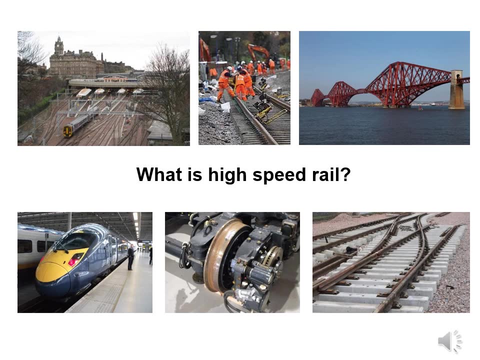 Now let's take a look at how specific a project is. It's a cyclone & nastier than we think, while it's definitely likely. So what is high-speed rail? In the next couple of slides, we're going to discuss some of the 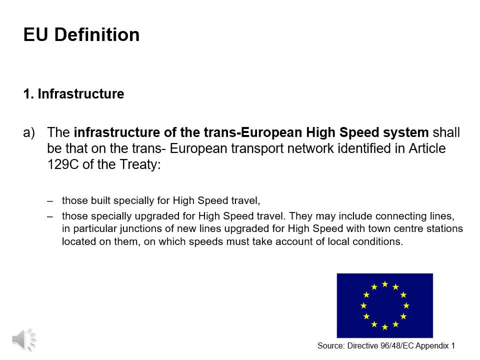 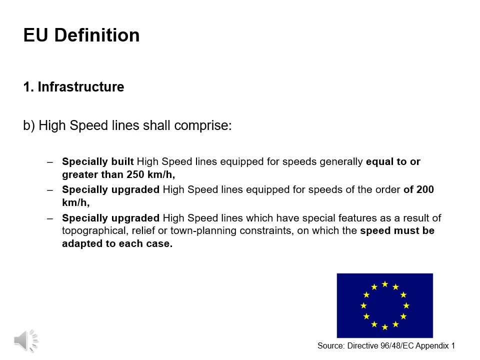 key definitions. So the European Union defines high-speed rail as the infrastructure of the trans-European high-speed system, those built specifically for high-speed travel or those specially upgraded for high-speed travel. So the EU definition then continues to define high-speed lines as specifically built for. 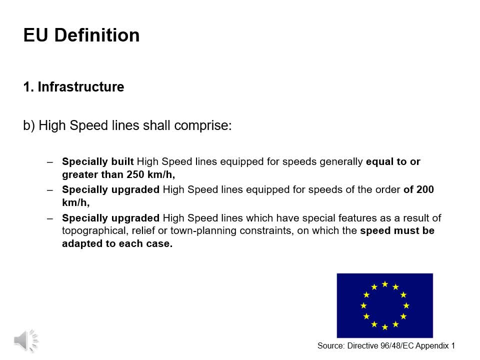 speeds equal to or greater than 250 kilometres per hour, specially upgraded with line speeds in the order of 200 kilometres an hour, or specially upgraded where speeds are adapted to each case. So the EU definition then continues to define high-speed lines as specifically built for. 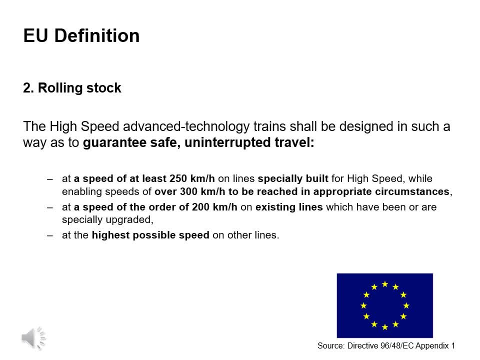 speeds equal to, or greater than, 250 kilometres an hour, or specially upgraded, where speeds are adapted to each case. So, in terms of rolling stock, the EU definition states that high-speed advanced technology trains shall be designed in such a way as to guarantee safe, uninterrupted travel. 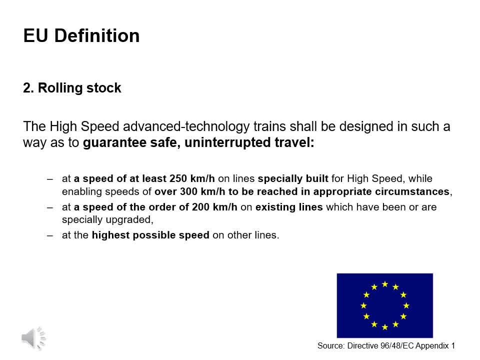 So they're going to be travelling at a speed of at least 250 kilometres per hour on lines specially built for high-speed, whilst enabling speeds of over 300 kilometres per hour to be reached in appropriate circumstances, a speed in the order of 200 kilometres per hour. to be reached, in appropriate circumstances, a speed in the order of 200 kilometres per hour at the speed limit. In a way, the EU definition eliminates that requirement as a course of time. It also demonstrates that high-speed trains are designed to achieve high speed, didn't. have to be blooming here and they're designed for higher speeds. So, on the EU definition, high-speed trains are designed to achieve at least 250 kilometres per hour or, specially upgraded, including in the order of 250 kilometres per hour. 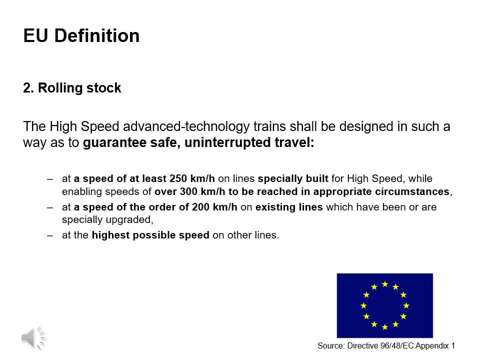 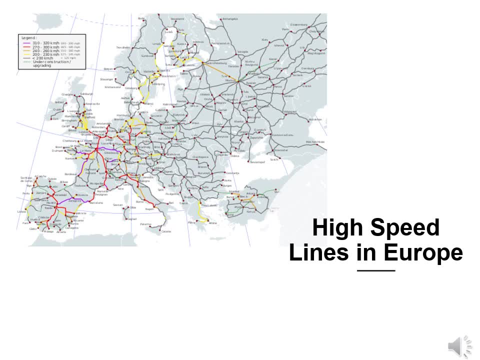 and at the highest possible speed on other lines. The EU definition then continues to define high-speed trains for high-speed travel and speed at the highest possible speed on other lines. So this map shows the high-speed railway lines across Europe. Note the legend: shows that the colours dictate the line speeds. 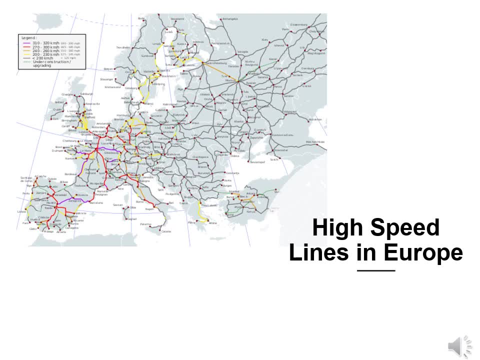 Note: the legend shows that the colours dictate the line speeds. Look at the purple lines in France and Spain, where you can see line speeds of between 310 and 320 kilometers per hour. That's around 190 to 200 miles per hour. 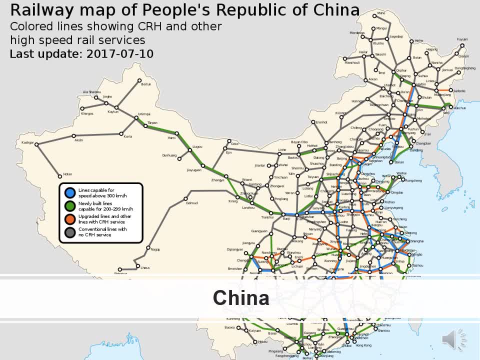 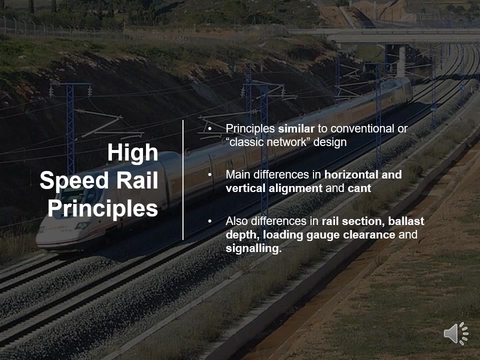 So, looking a bit further afield now, the People's Republic of China have developed their high speed rail capability significantly over the last few years. Here you can see a map of China and pay particular attention to the blue lines where we see line speeds capable for speeds above 300 kilometers per hour. 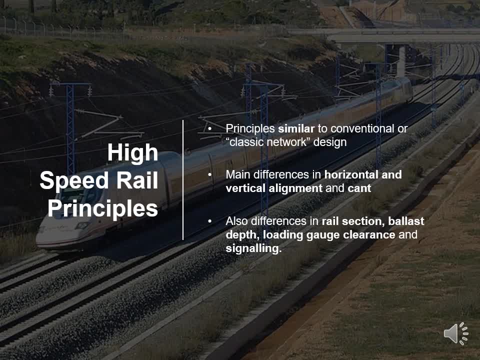 So, in summary, there are three high speed rail principles. The first one is that they're generally similar to conventional or classic network design. The main differences are in horizontal and vertical alignment and increased cant. Also, there are differences in the rail section, the ballast depth, the loading gauge clearance and the signaling systems that are adopted. 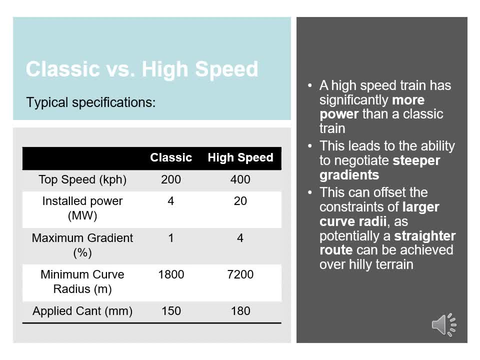 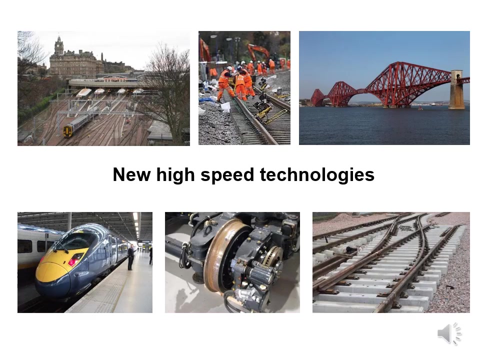 This slide compares some of the typical specifications for classic versus high speed rail. A high speed train has significantly more power Than a classic train or locomotive. This leads to the ability to negotiate steeper gradients. This can offset the constraints of larger curve radii, as potentially a straighter route can be achieved over hilly terrain. 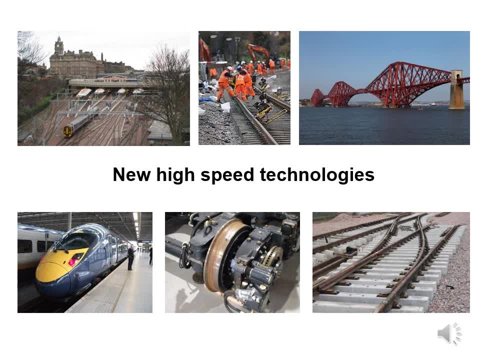 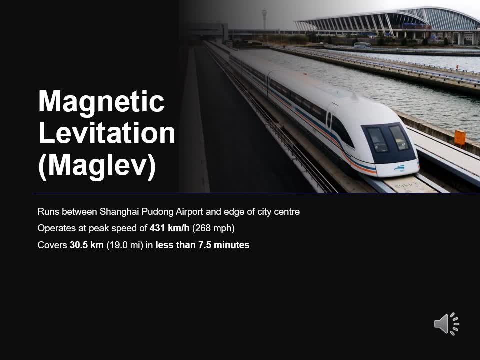 So I'm going to end this lecture with a look at some of the new high speed rail technologies that exist in the world. The People's Republic of China Have the world's first Passenger Carrying Operational Magnetic Levitation Railway, otherwise known as a Maglev train. 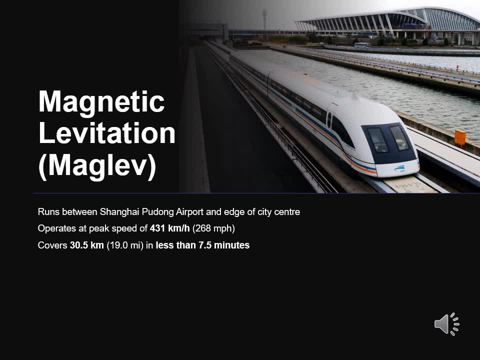 It runs between Shanghai Hunong Airport and the edge of the city center. It operates at peak speed of 431 kilometers per hour, That's 268 miles per hour. It covers 30.5 kilometers in less than 7.5 minutes. 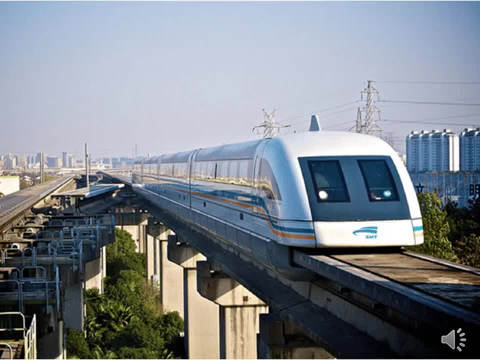 The people's Republic of China Have the world's first Passenger Carrying Operational Magnetic Levitation Railway, otherwise known as a Maglev train. It runs between Shanghai Hunong Airport and the edge of the city center. It operates at peak speed of 431 kilometers per hour. 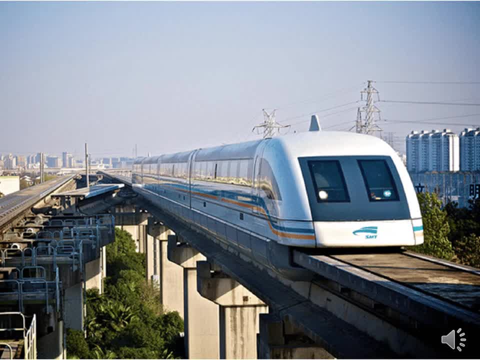 That's 268 miles per hour. That's 268 miles per hour. The people's Republic of China Have the world's first Passenger Carrying Operational Magnetic Levitation Railway. otherwise known as a Maglev train, It operates at peak speed of 431 kilometers per hour. 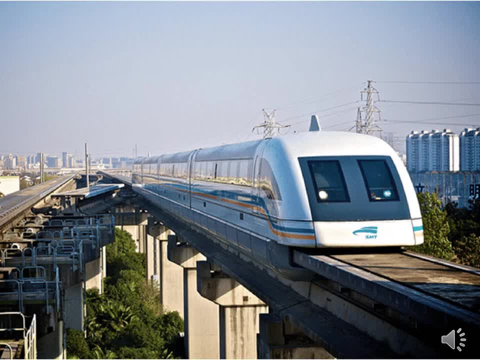 That's 268 miles per hour. That's 268 miles per hour. The people's Republic of China Have the world's first Passenger Carrying Operational Magnetic Levitation Railway. otherwise known as a Maglev train, It operates at peak speed of 431 kilometers per hour. 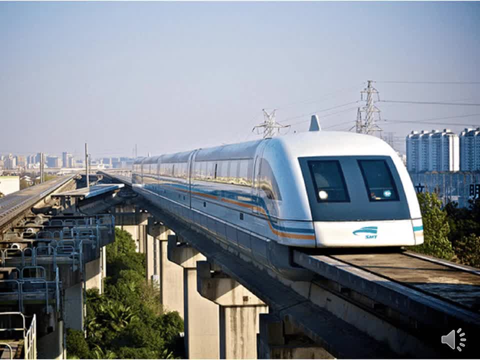 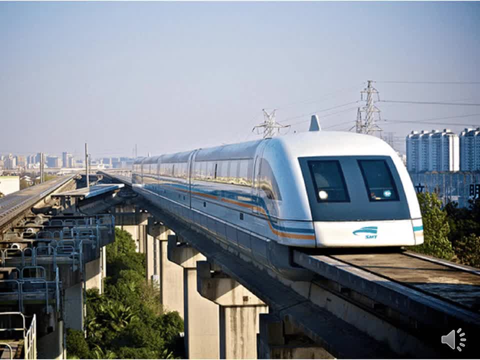 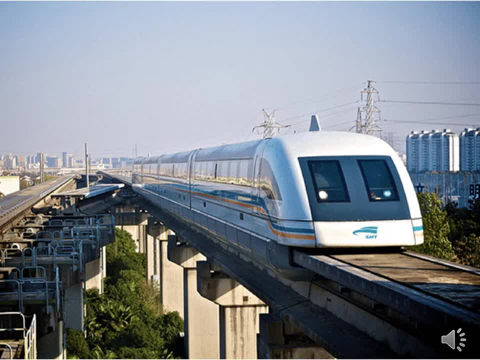 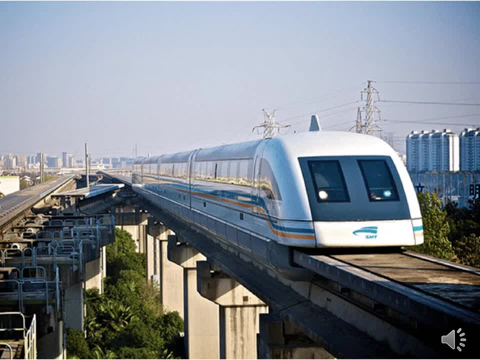 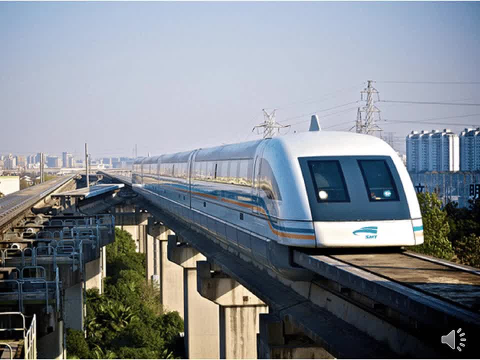 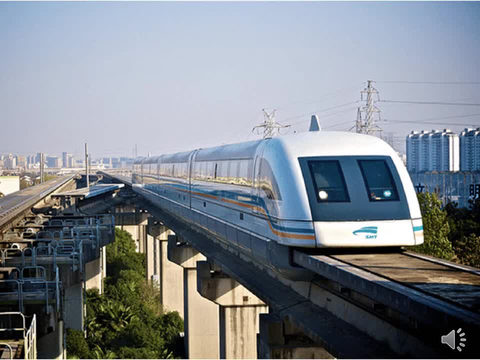 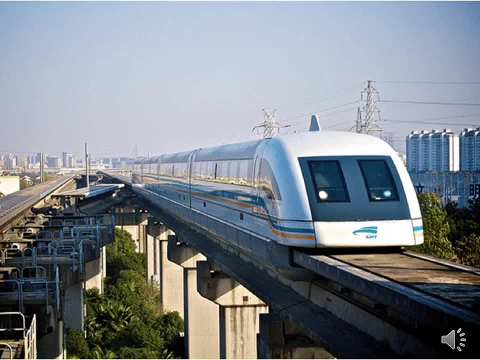 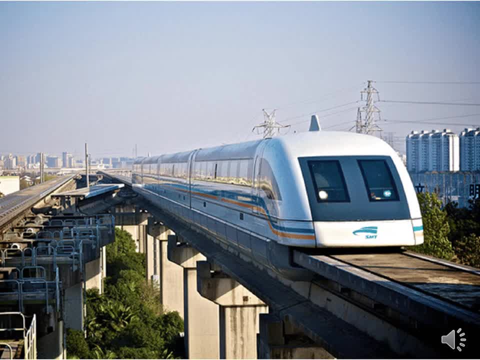 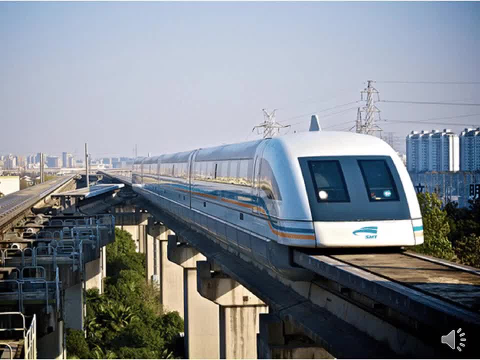 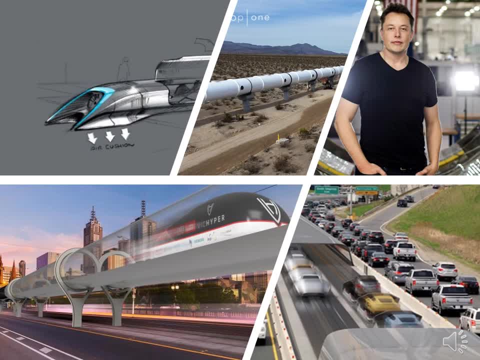 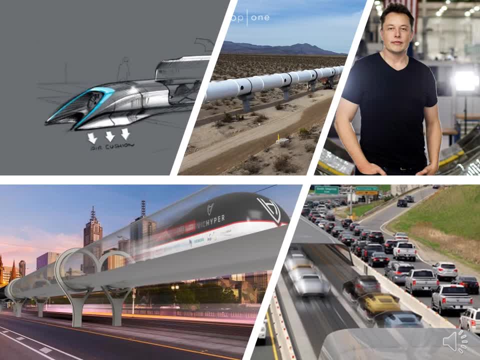 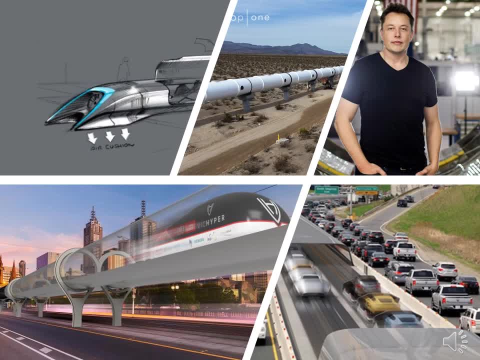 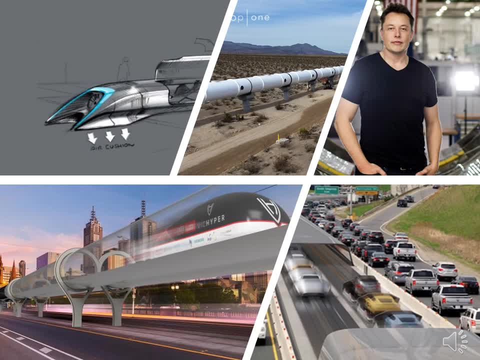 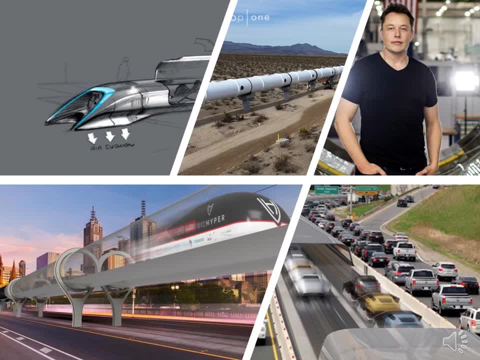 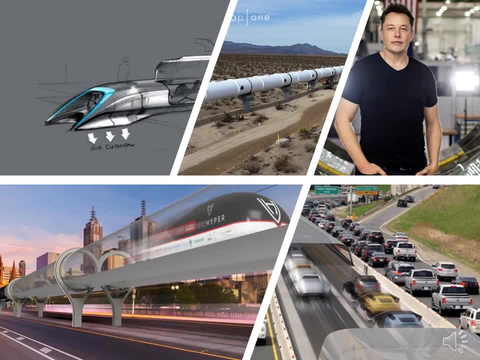 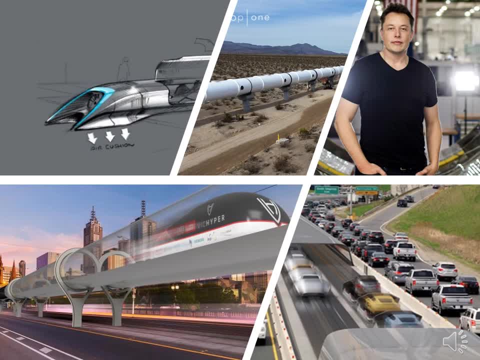 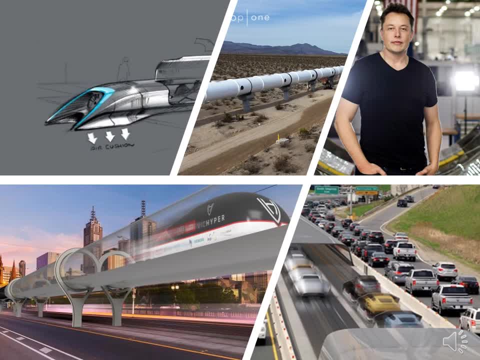 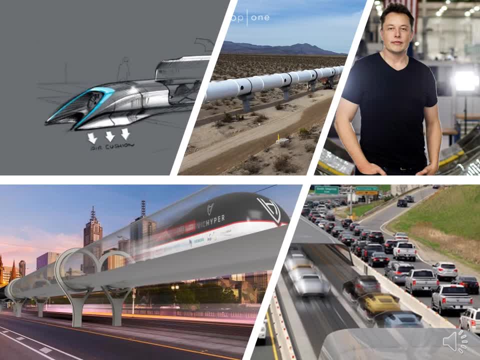 That's 268 miles per hour. I don't know. I'll let you guys have a think about that and you can post your thoughts in the discussion forum. The next couple of slides: I'm going to look at some of the world's fastest conventional. 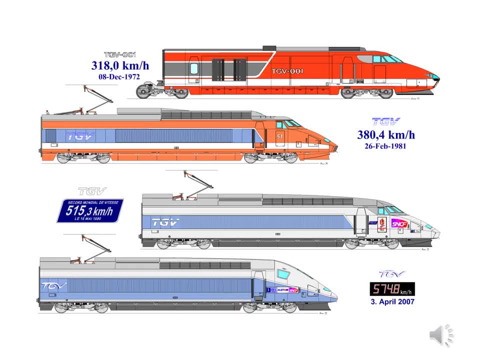 trains. I'm going to start off with the French TGV. In December 1972, about four years before I was born, the TGV 001 was running its speeds up to 318 kilometers per hour. By 1981, it was reaching speeds up to 380 km per hour. 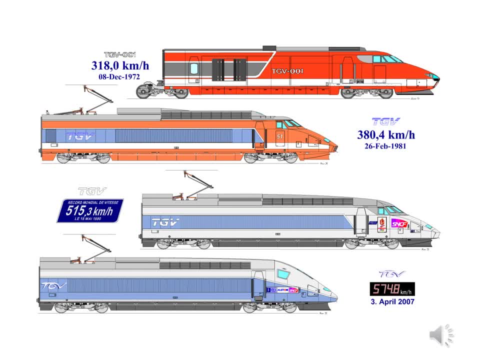 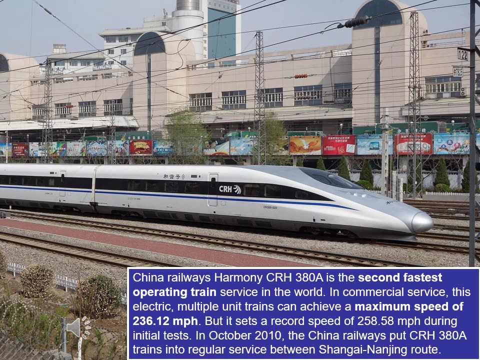 By 1990, we're seeing the TJB running at speeds of 515 km per hour, And then in 2007 it was hitting speeds of 574 km per hour. In China, the Harmony CRH380A is the second fastest operating train service in the world.